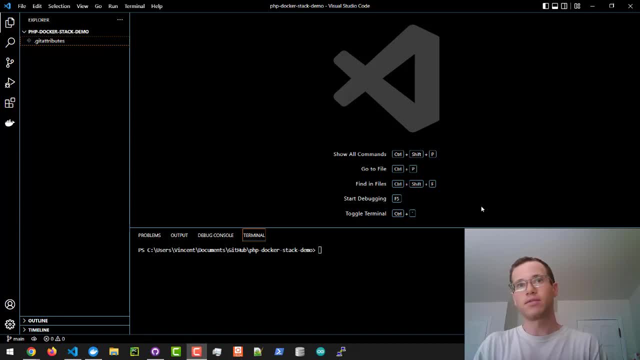 if it's a Windows machine or a Mac or a Linux based operating system, it will run the same, no matter where else you go. It makes deploying the products that you make as a web developer a lot easier and faster. So we'll jump into how you do that in this video. And PHP is. 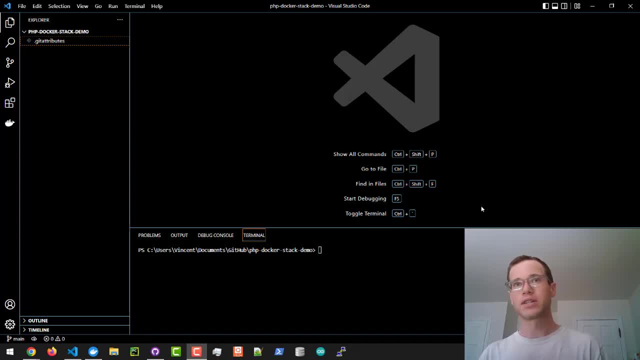 an old language, but there's been a lot of iterations and versions to it that still keep it a fairly fresh and modern language to use when you're writing a website. So a very great way to jump into the full stack of web development, and that's why I'm really excited to share. 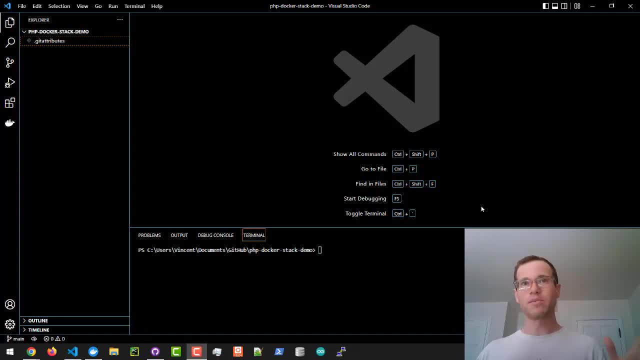 with you guys this stuff. So I have an empty project repo in front of me and we're going to be walking through the steps to create this entire full stack web application, from the PHP to the MySQL database, as well as the actual images that are going to be running. 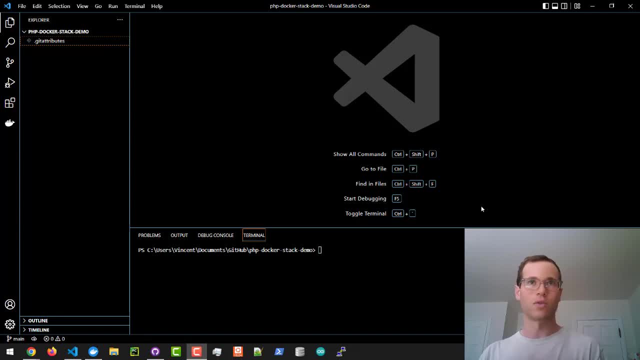 their operating systems so we can run an Apache web server to handle these requests that we get for users who want to view our website. So the very first thing I'm going to do is I'm going to right click in this folder I have, I'm going to create a new file and call: 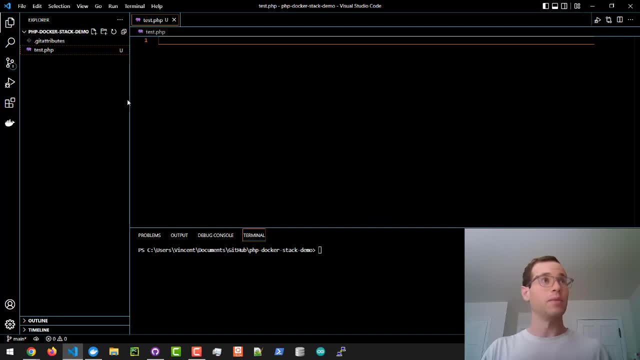 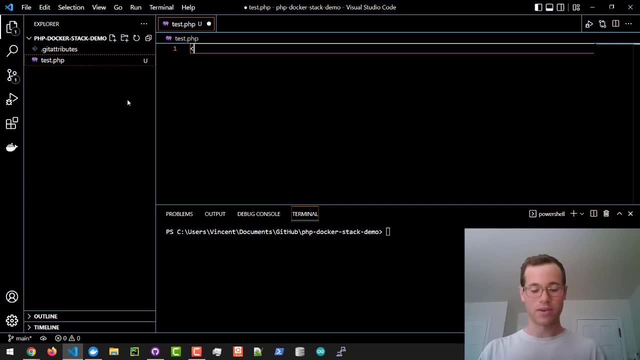 this testphp- And I'm going to try to make this bigger for you guys, because I can't see that well either- And basically what I'm going to do here is I'm going to just write up some very simple PHP And all it's going to do is echo: hello world. and you always need to remember that semicolon. 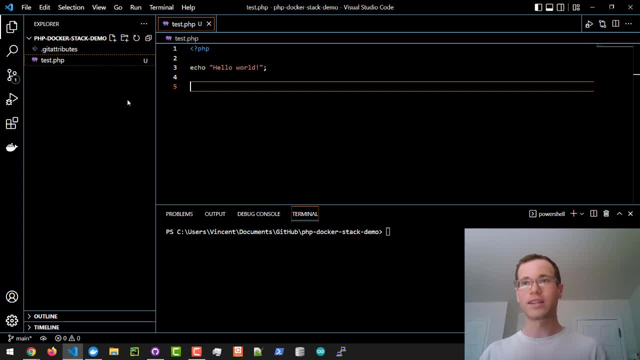 to end it, and then you're going to press control save on the keyboard, And so, just like that, I have created a little PHP file, but I can't view this page in a browser. It's not able to be rendered. So what I want to do is I want to create a new file inside of this project. 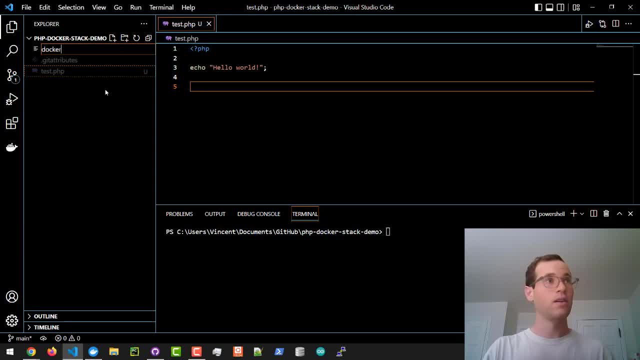 and I'm going to call this docker-composephp, And the purpose of this file is going to be telling docker what images does it need to grab in order to make this thing run, and you can define some other properties that we will be doing in just a moment. So the very first thing inside of your docker-compose file is: 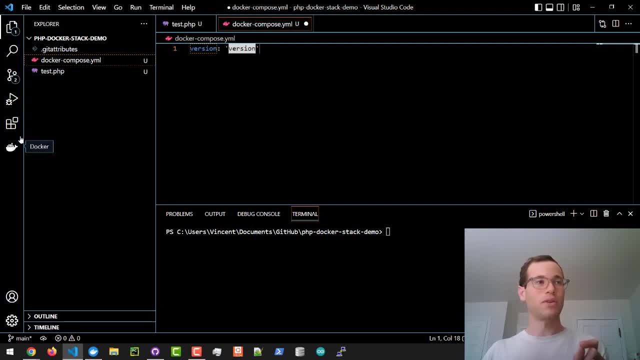 going to be the version And if you have installed the docker plugin. I'm using VS code. there is a docker extension for VS code that enables this kind of autocomplete. that makes it really slick for when you're doing this stuff, Like I didn't have to finish typing. 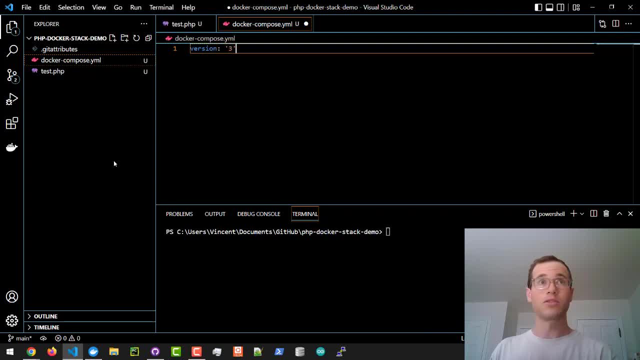 But I do recommend installing that if you're getting into this. So we're going to be going with docker version 3.. And I can just add a comment by doing a little hash like that: This is the docker version And then a newline character. You don't need to worry about commas. 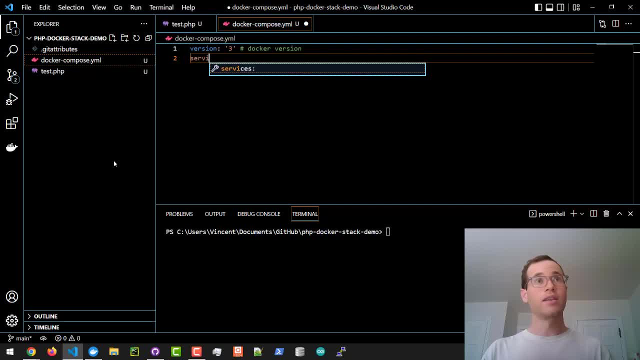 or semicolons with yamls, And then we're going to be defining the services that are going to be associated with this docker container or container cluster as we'll refer to it. So, basically, inside of our services- this is where I'm going to say- we're going to have 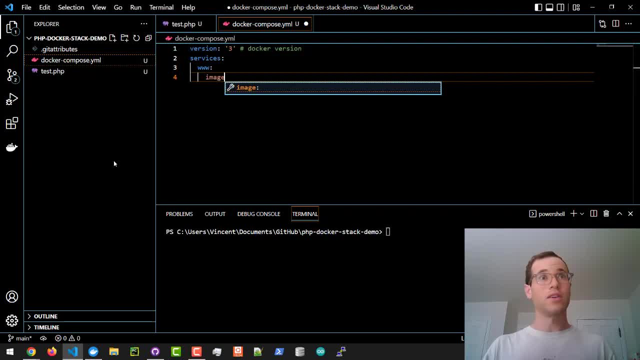 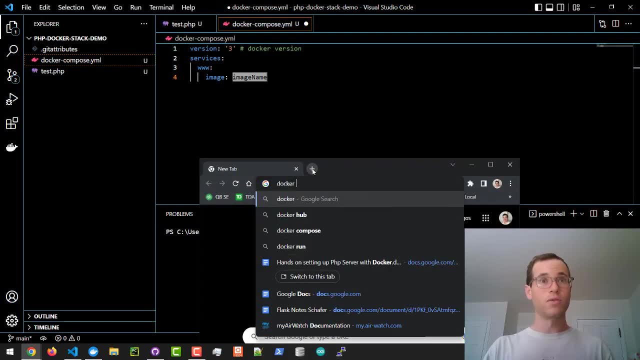 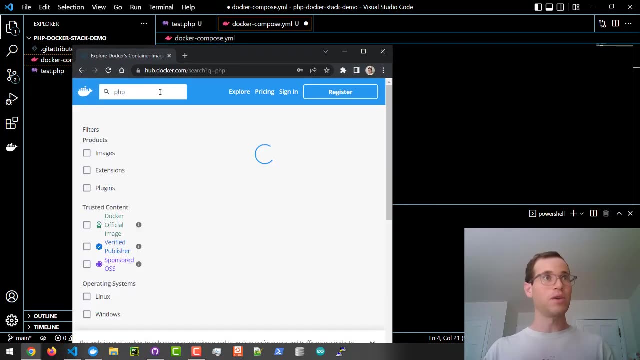 a www service And it's going to have an image, And we have to give this an image name. This image name comes from the docker hub repo, So if you google docker hub, you can click on here and it takes you to the website, And so what we want is a PHP image, because 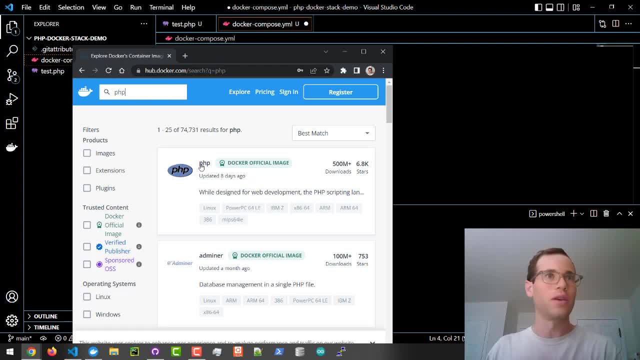 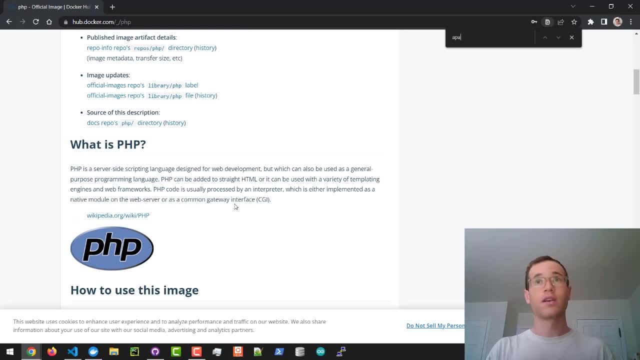 we're going to need a container to handle running our PHP code And specifically, what I want in here is the one for Apache. So I'm just going to control F Apache And you can see that you will eventually get to a point here where they're telling. 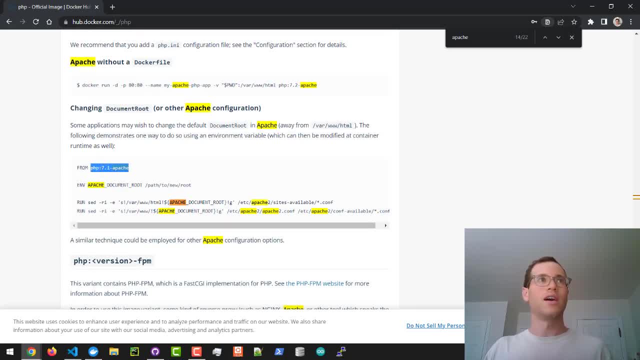 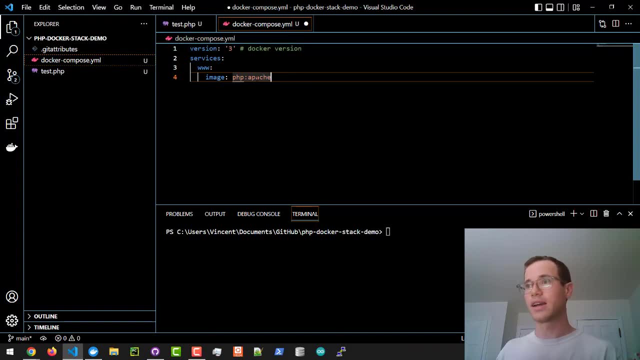 you PHP versions that have Apache in them. I'm going to be just going with the latest thing here, So I'm going to close this out And so, basically, it's going to be php//apache, just like that, in order to define the image that we'll be using for this particular service. 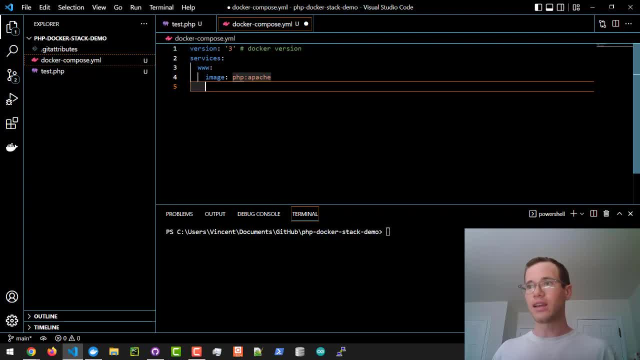 in our full stack web application And I'm also going to be defining volumes like this, And the purpose of volumes is to sync- have a two way real time sync connection between your running container and your local host And you need this so that, whatever you're- 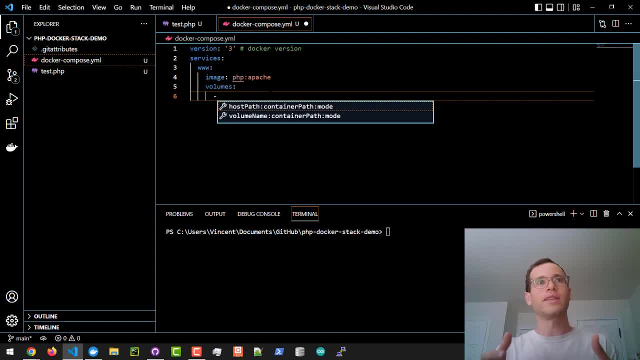 writing inside of VS code right now is on your local machine. You want this to be synced with your container so that your container will reflect the new PHP code that you're writing into it. So what we're going to say is that I want to sync and you'll space, and then you'll do. 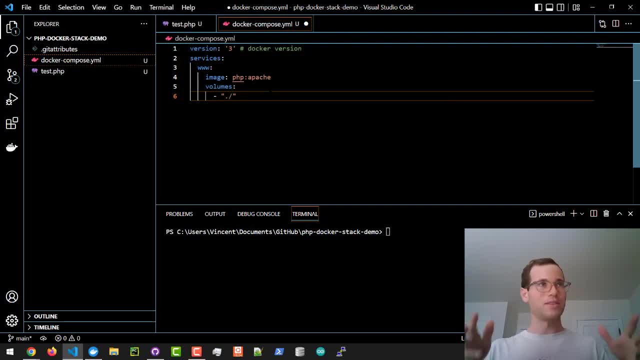 a double quotes dot slash. That basically means the current directories. that is, the project directory we are currently in- And I want to sync this with this- is now on the container side And this container is going to be running a Linux operating system. So 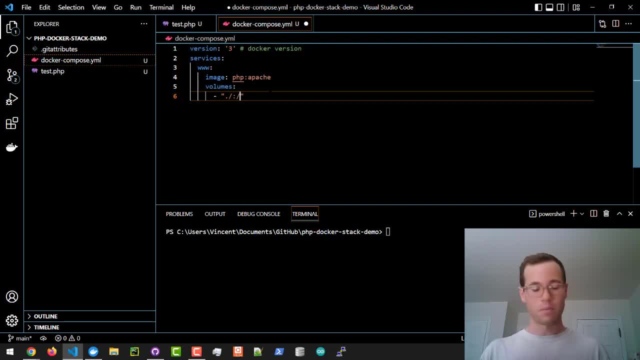 if you're using, if you're familiar with Windows paths, it'll look a little bit different, But it's var wwwhtml, So basically everything you see in here will exist inside of the container under that volume, And I'm just going to specify that. So sync projecter. 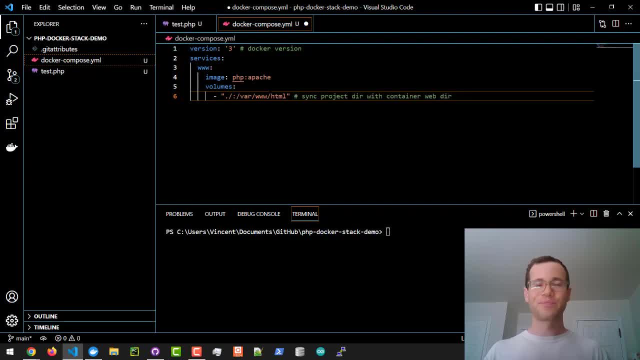 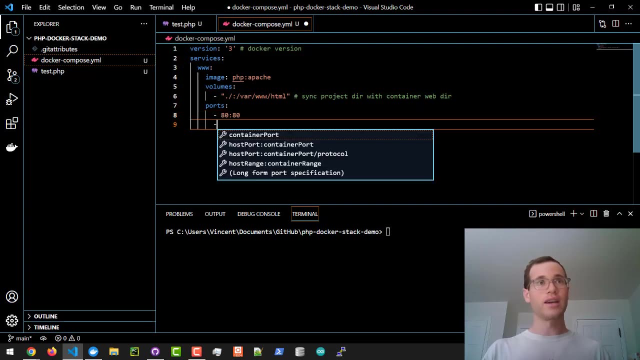 With container web dir And I'm going to also want to specify the ports here. And specifically I'm going to be binding port 80 on my local machine to port 80 of the container And in addition to that, if we ever wanted to serve SSL stuff, we will be finding port 443 as. 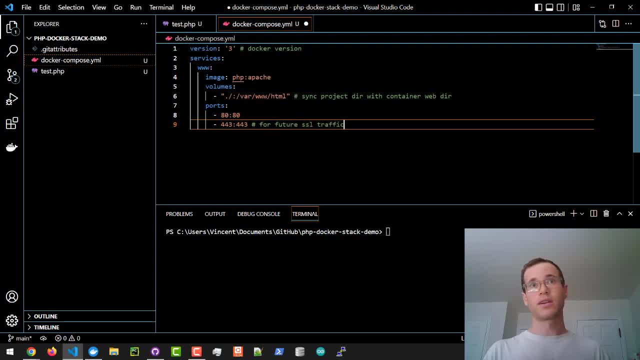 well. So this is just for future SSL traffic. just you have a little bit of. you can add some security Down the road. I'm going to now press control save on the keyboard, or command save if you're on a Mac, And now what we're going to do is inside of VS code. they're really cool at. 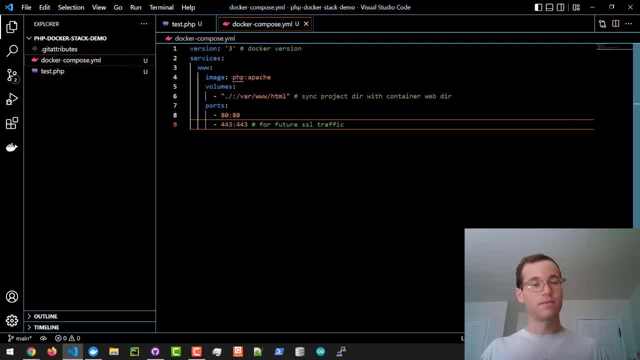 showing you a terminal. So if you press command or control tilde pulls up this terminal right inside of your project repo. And what I'm going to do is I'm going to run the command at Docker dash, compose up, And so when I run this guy, what it's going to do is it's going. 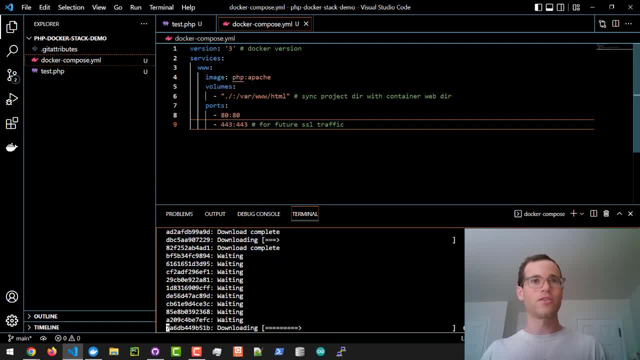 to find the Docker compose YAML file inside of my project directory. And then it's going to say, okay, I need to get this PHP Apache image that's been specified. it doesn't have it, So now it's going to run through actually downloading all the stuff. 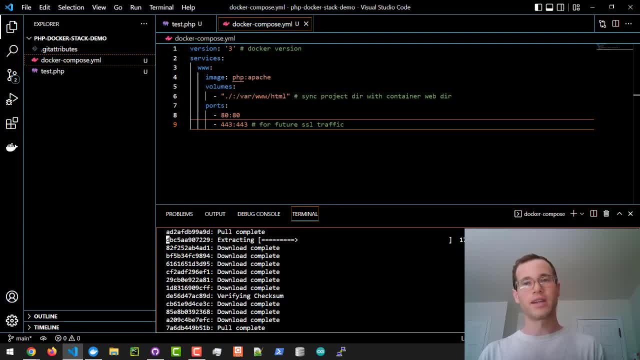 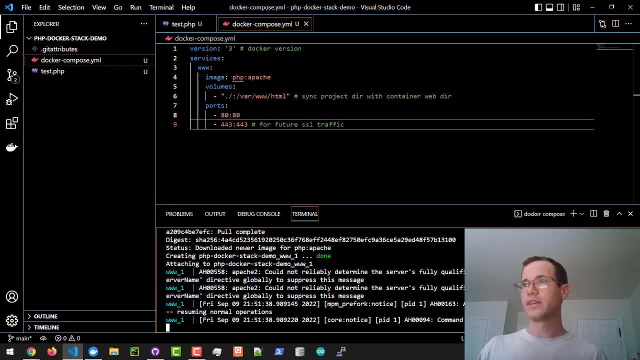 that it needs to do this, So we will give it a moment to do all that, And it can take some time, So I'm going to let this thing speed on through, All right. And so the other thing to note is that once this thing finishes doing this, I do recommend opening up Docker. 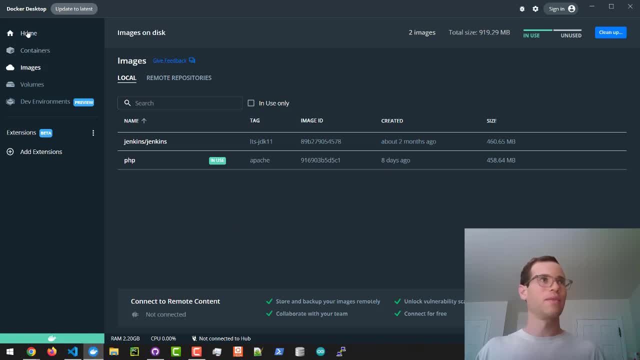 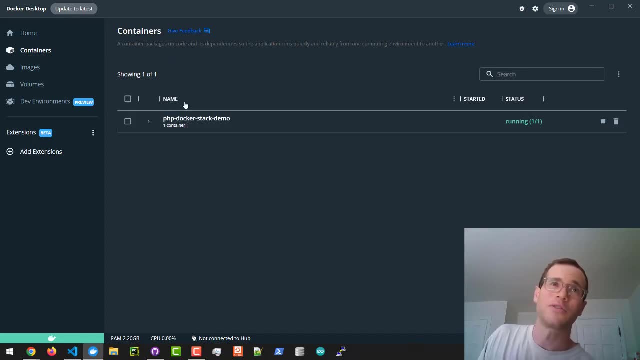 desktop If you're running this on like a on a Windows computer or Mac, whatever. If you click on containers, you'll see that it has now created this thing: PHP Docker stack demo. So it's referencing your project name in it, So it'll reflect whatever you've named. 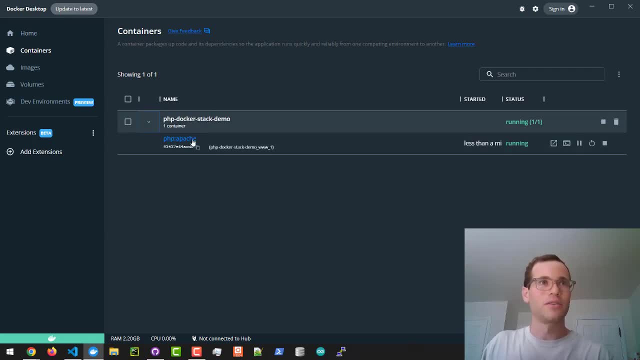 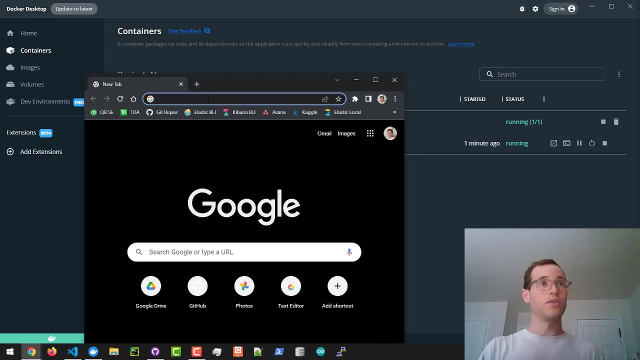 your, your parent directory, And then, if you click this, you'll see that it now has a little container spinning for us and it's running, which is great. So what I'm going to do is I'm going to open up a new tab in Windows And I'm just going to go to localhost port. 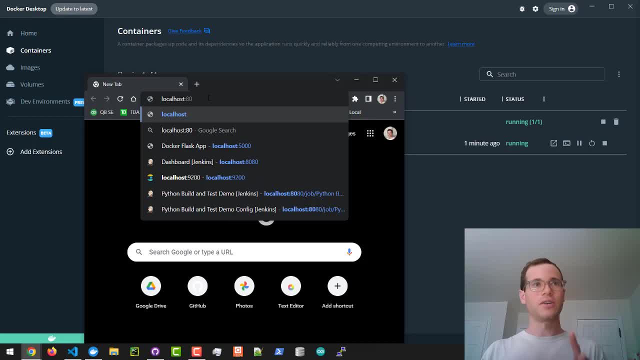 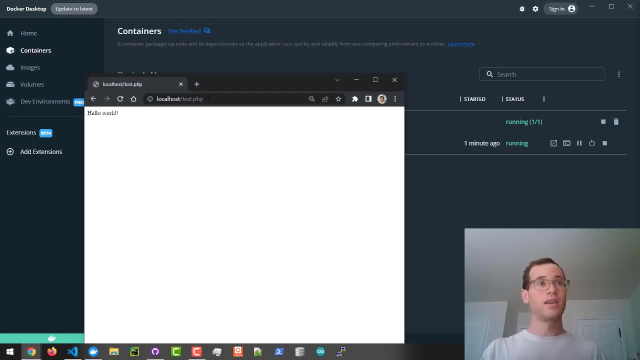 80. And it's important to know that this is actually the default port, So you can just go to localhost itself And don't need to specify the port. but then you do a forward slash And specifically in our case I call that file test dot PHP. So I'm just going to type that in. And now 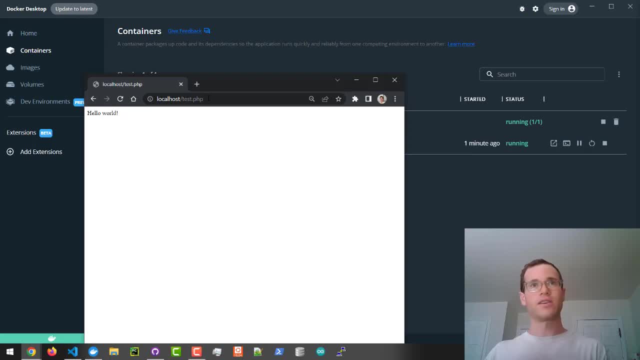 we have a web server running inside of a Docker container on our host machine, in this case a Windows machine, And it is returning us traffic when I send a get request to port 80 on it And you can be really explicit if you want. So you can have like a port 80 there It's. 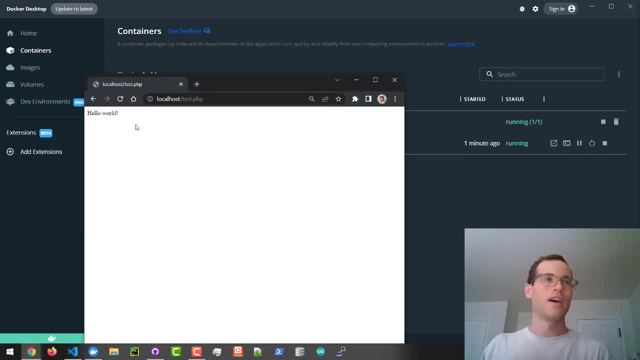 going to be the exact same thing, And Chrome even truncates it for you, But that is how we get the PHP service up and running. It's not really a full stack web app, though, because we don't have a database. We're not connecting to a database, So we're going to want to improve. 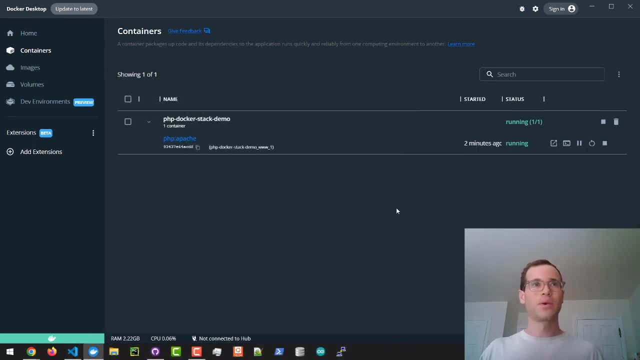 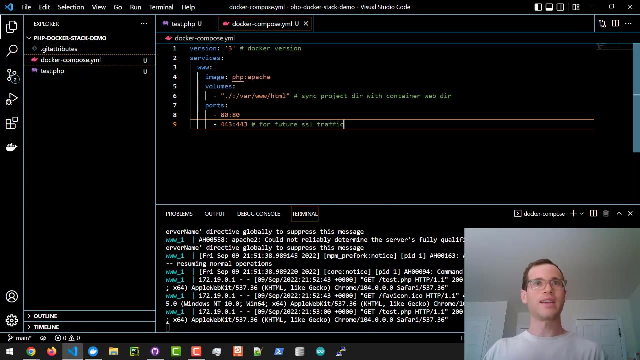 this and add some features to it, Right? So I'm going to close this guy up and I'm going to go back to VSCode, And what we're going to want to do is we're basically going to be adding an additional service into our database. 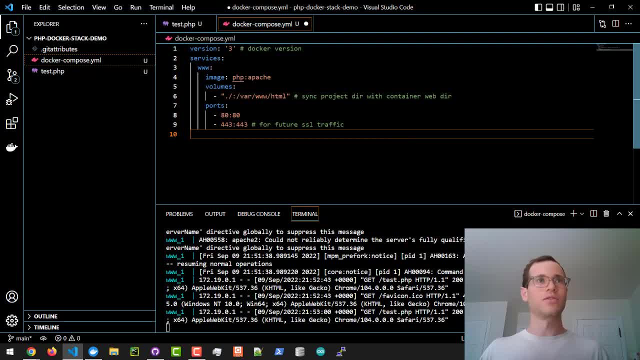 Docker compose file. So we've got the WWW service right here. I'm going to close that up or minimize it. I'm also going to have a DB service to be our database And I'm going to specify the image and the image name specifically. This is stuff you get off of MySQL Hub, or you. 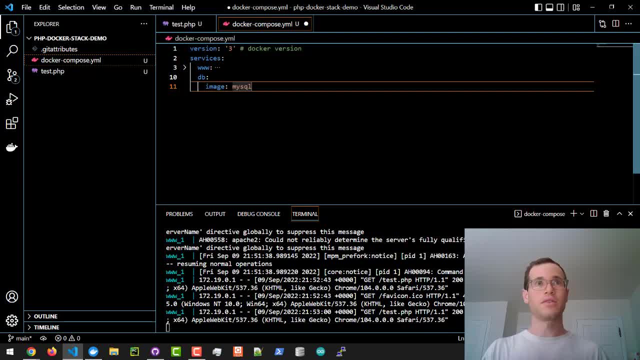 can just copy it from someone else. This is going to be MySQL colon latest, So it's just going to pull the latest version of MySQL from Docker, So you don't have to worry about downloading stuff manually. And then you're also going to be defining the name of the server, So you're going to want to 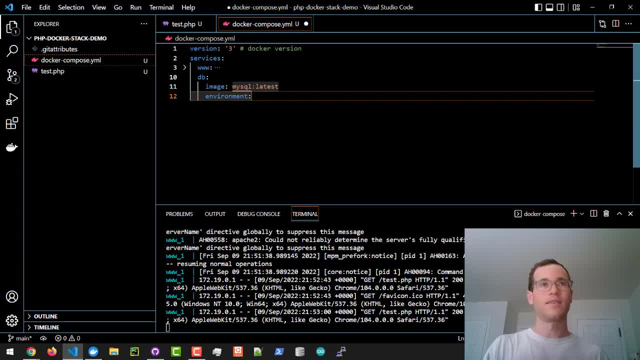 define some environment variables for this particular image. So in our case, I'm going to paste in some stuff just to save some time. I'm just going to paste that guy in just like that, And you need to get that spacing just right, otherwise it complains. 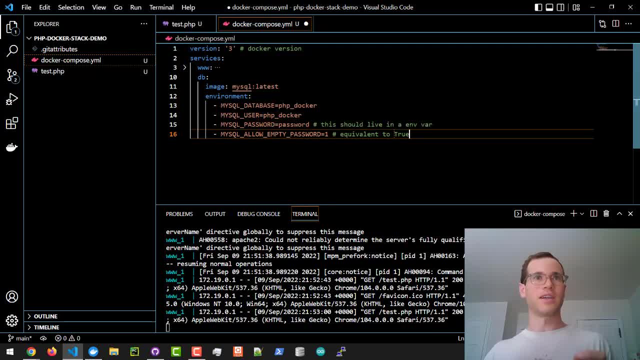 But yeah. So what we're doing here is we're going to be specifying the database name, as well as a user for this database and a password, And we're also going to be allowing to have an empty password, just so it doesn't complain at us. but now that we have added a 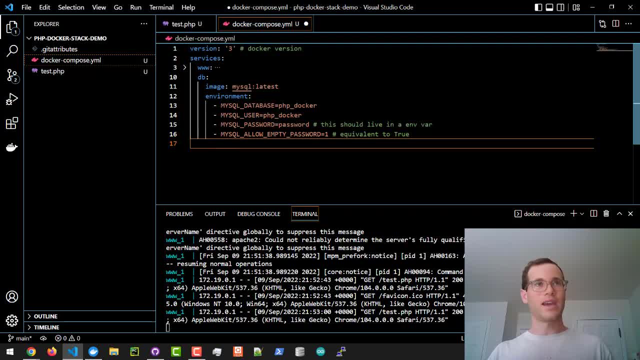 database service. I also want to add a service to have a web interface to look at this MySQL database. we're spinning up, so in that case, what I'm going to be doing is also adding another service in here, which I'll just copy paste in. you guys can copy this right off of GitHub. 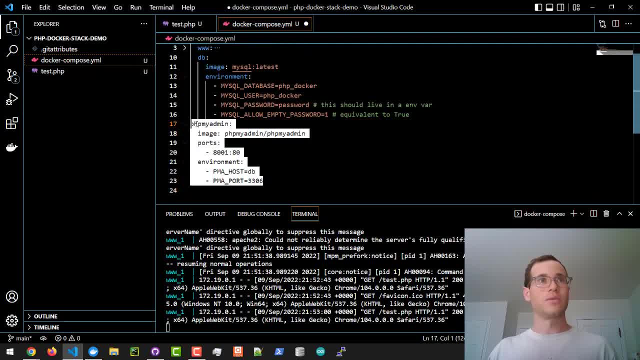 we're just going to paste that guy in and make sure that we get our indenting right. so basically what we're doing is we are grabbing the php myadmin image off of docker hub as well, and then we're going to be binding port 8001 on my local computer to port 80 of the actual 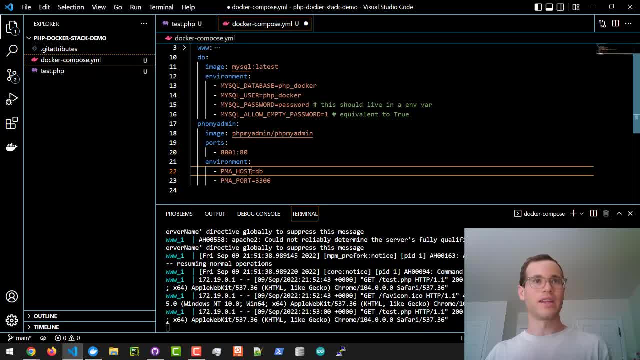 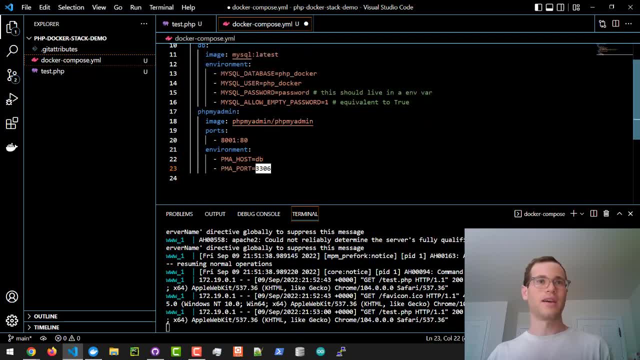 container itself, and then we're also defining the name of the service for the php myadmin or pma to grab, as well as the port that it should be working with. so in that case it's 3306, which is a default value for myadmin. 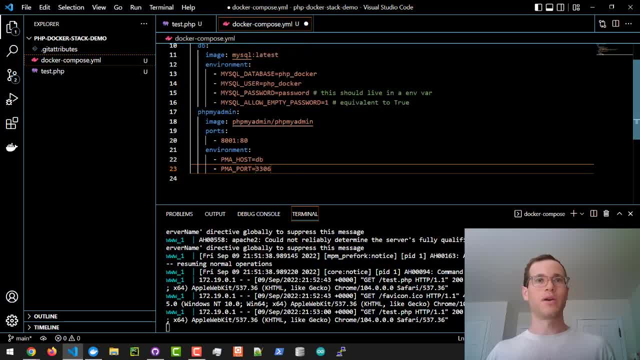 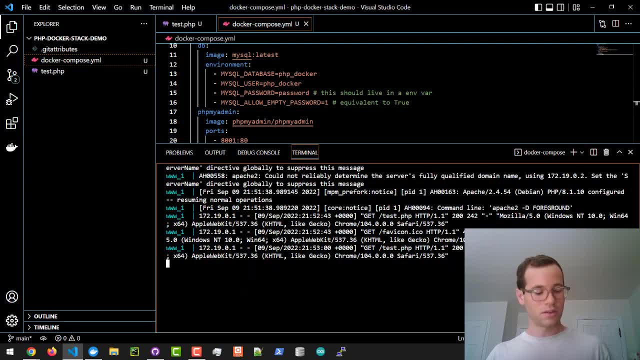 MySQL. so we've now updated our docker compose file. I'm going to press command s to save. I'm going to go to my terminal right here, I'm going to press ctrl c and this is going to stop the running containers, and I'm also going to run the command at docker dash compose down like that: 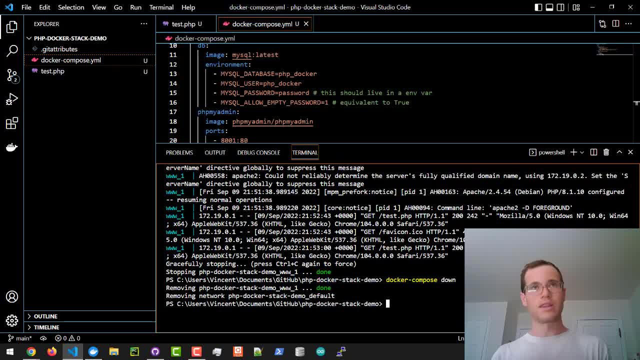 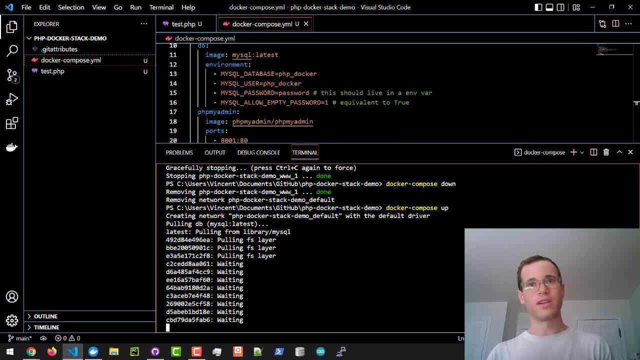 and it's going to have the effect of basically stopping everything that was going on. and I'm going to run the command of docker compose up just like this. and now, when we're restarting our docker compose file, we're going to run the command of docker compose up just like this, and: 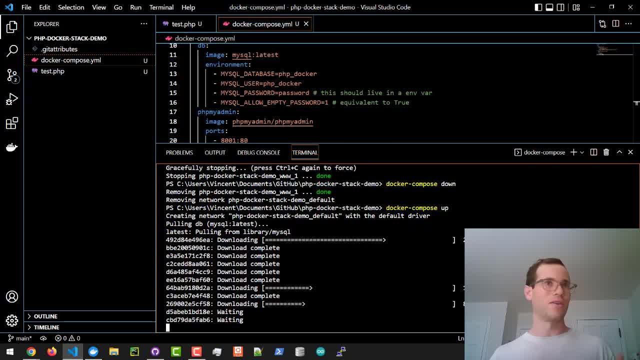 now, when we're restarting our service, it's going to realize that it doesn't have all the images that it needs, so it's going to run through the process of downloading the mysql image as well as the php myadmin image from docker hub, and so we'll let this thing run through and then we'll get back. 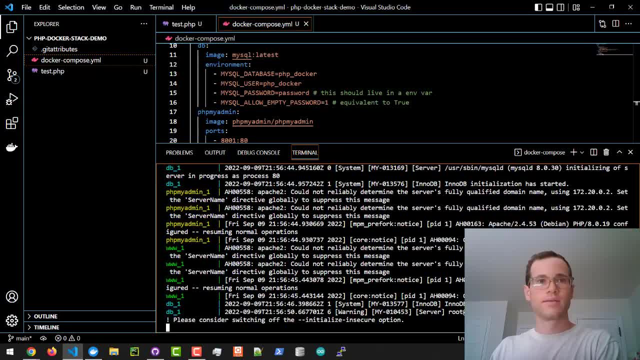 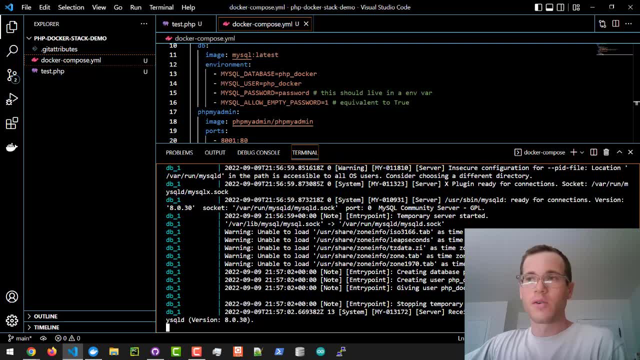 to it. all right, so it looks like it has finished downloading these things, and now these are logs just from the services that are coming up online. one thing I do want to call out now is that if you go to docker desktop again, you won't be able to see any of the things that are coming up online. 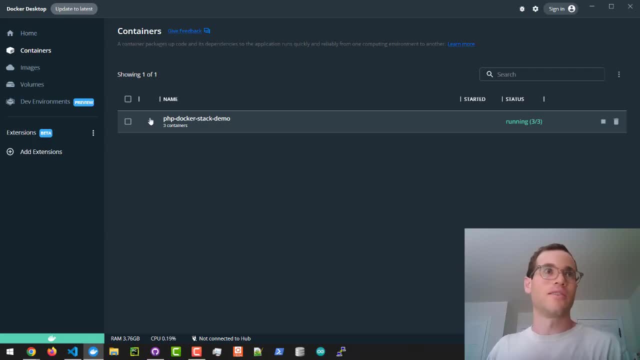 you will now see that, our little cluster of containers. there's now three of them in here. so we've got the mysql service, we've got the php service and then we also have the php myadmin service, which is what lets us have a nice ui to our mysql database service that's running now in. 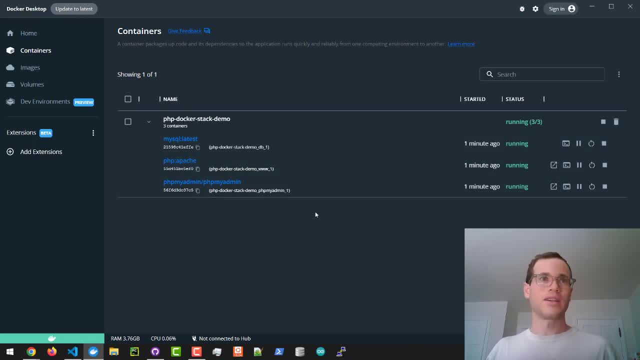 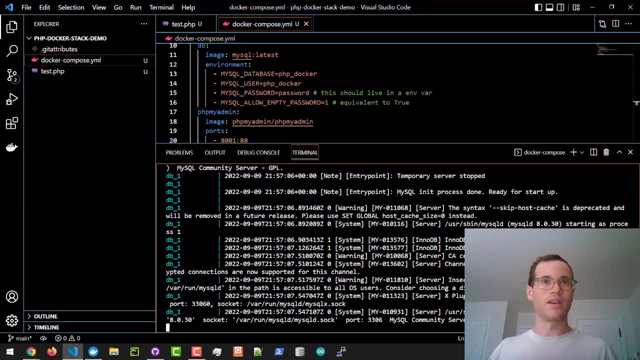 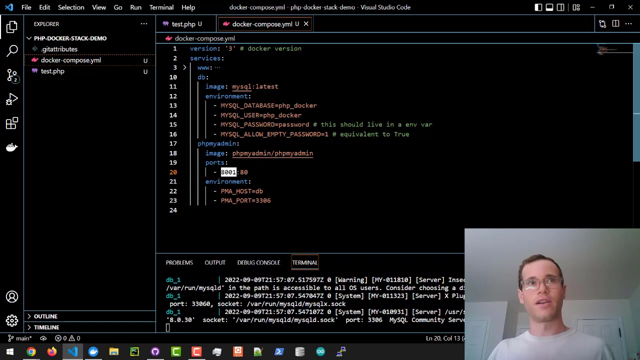 our container. so these things are all running, which is great, and now what I'm going to do is I'm going to open up another window right here and I'm going to go to. so if we recall in our in our docker file right here, that we found port 8001 on our host to port 80 of this container. so I'm going to go to localhost and 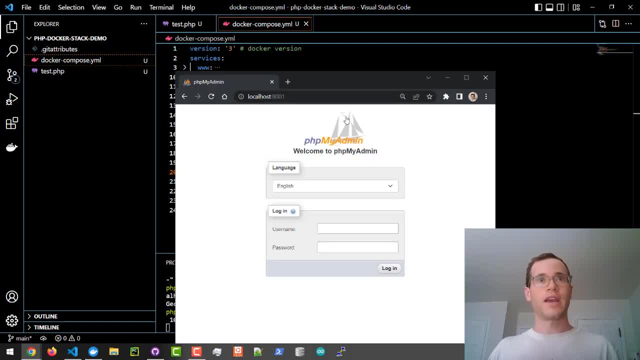 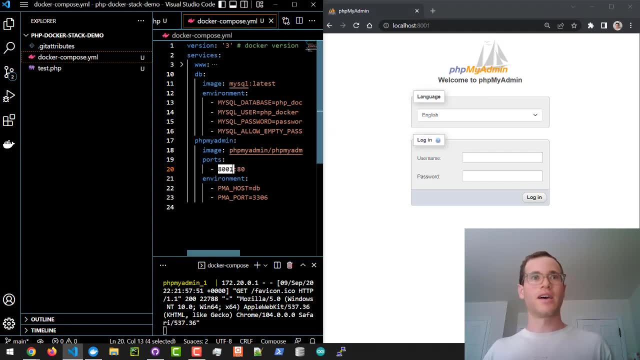 instead of port 5000, I'm going to go to 8001 and you can see that it now takes us to this login page. and so, on this login page, when you do that, it is prompting us to put in the username and password, and the username and password for this is what we've defined already for the mysql service. 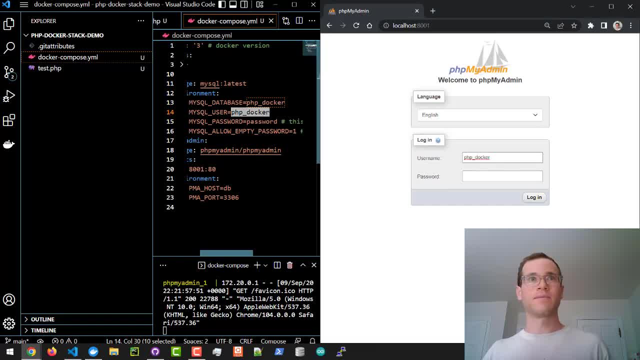 which in this case, was just php, my docker or, I'm sorry, php docker- and then the password was password. obviously, if this is a production environment, you should put this into an environment variable. you should have a much more complicated password, but for the sake of this little demo, this is where we're storing. it is just. 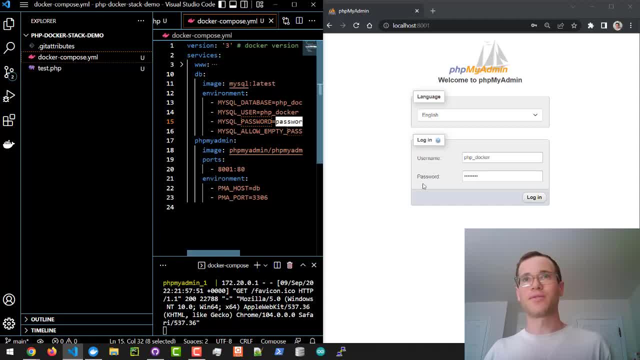 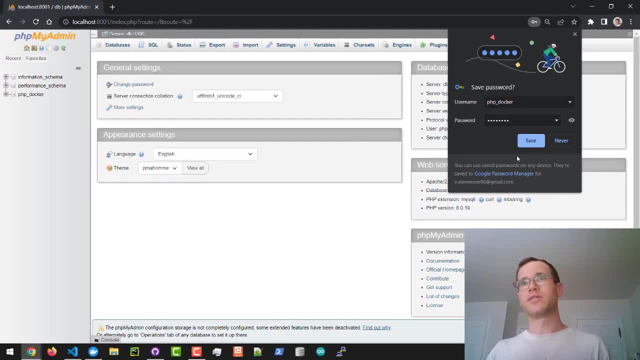 naked plain text inside of our docker compose yaml file. so just put on these creds. I'm going to click login and it's going to now authenticate me. I'm going to save these creds just so I don't have to always remember to punch them in. but if you want to save them, you can do that by clicking on the. 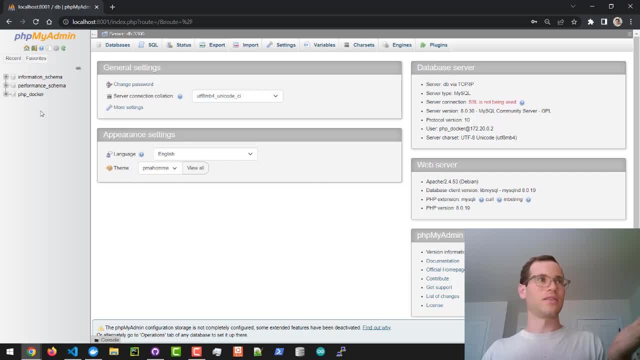 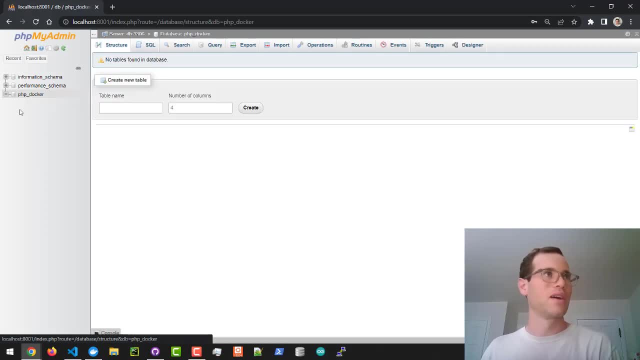 first one. you can do that, but now that we've done all this, you can see in the left pane that it's showing us these databases that exist. we care about that php docker database because that's the one that we've created for our specific web app. I'm going to click on it and it's going to tell. us that we don't have any tables, so we need to make a table inside of our database itself, and in our case, I'm going to call this table php underscore, docker table, and we're going to give it four columns and click on create, and so this is where having a little bit of knowledge of php helps. 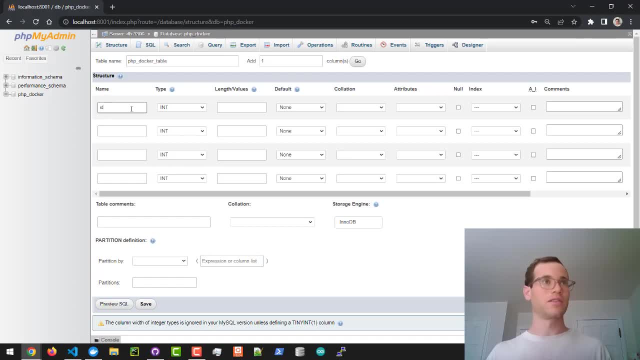 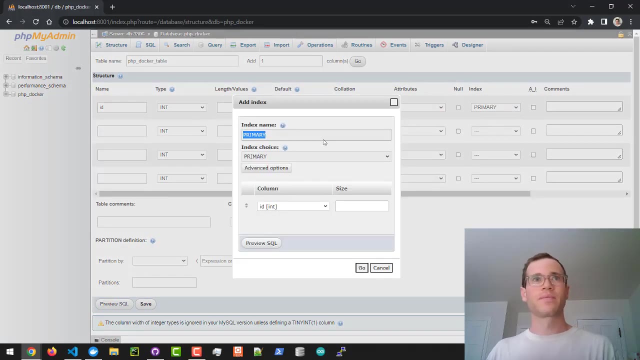 sorry of SQL helps, But for the sake of just getting started, we're going to give this one thing. It's going to be called ID And ID is going to be the primary key. So there's a thing in here where you define it as the primary key and click on go. So your database needs a. 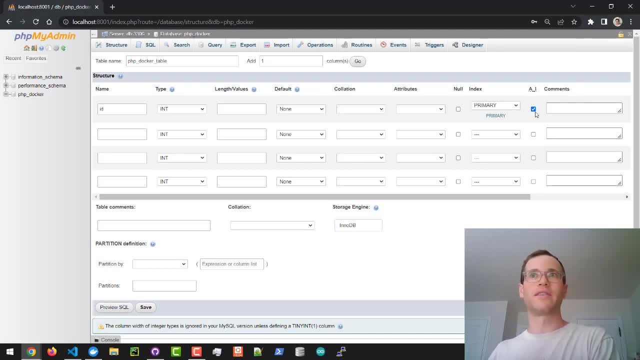 primary key for SQL. And then this AI thing means auto increment, And you do want your primary key to auto increment, because every single row inside of this database needs to have a unique primary key, Otherwise it will have a lot of issues. So you need to check this regardless of whatever. 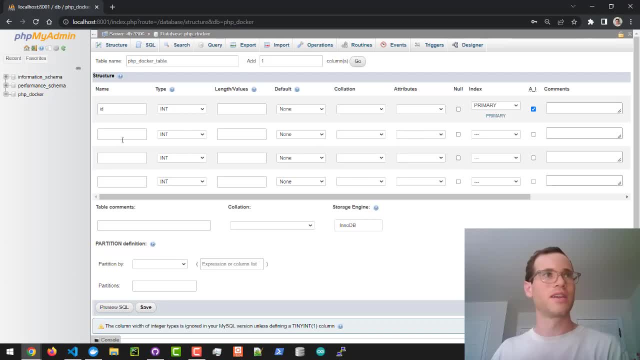 kind of database you're making. You need to have that as long as it's SQL database. And then the next thing is I'll say I want to add some things into my database that'll have some kind of title. So if this was a bunch of little blog posts, these things would have titles And the title 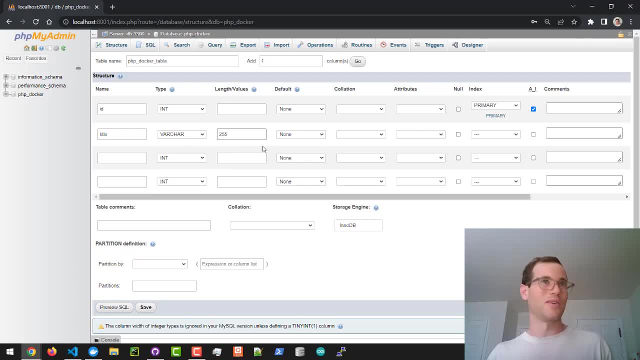 is usually a shorter string. So I'll say titles can be up to 255 characters in length. And I also would say: you know, my little blog posts would have like a body, And the body is going to be a series of text. you know some sentences or whatever, And then I'm also going. 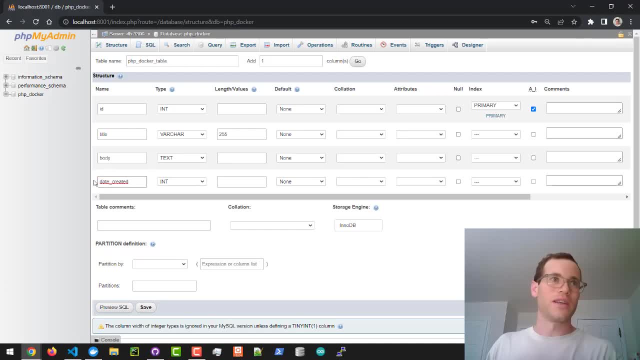 to have a day created property in my thing And I'm going to call this a text type of an attribute for my SQL database And the other thing is that's it, So you can try to have it default to current timestamp. I was running systems. 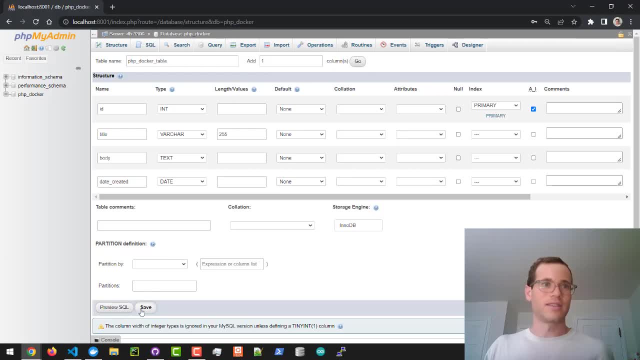 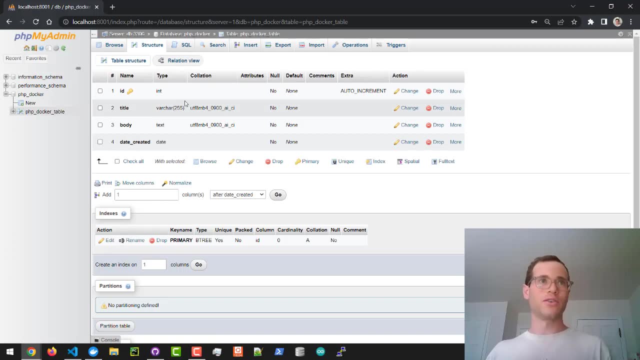 I don't have any issues with this, but I'm just going to click on save, And you can see that it has now created a table inside of our database, which is awesome. The next thing, though, we want to do is we want to put some data into this thing, just so we can show how to connect to a little. 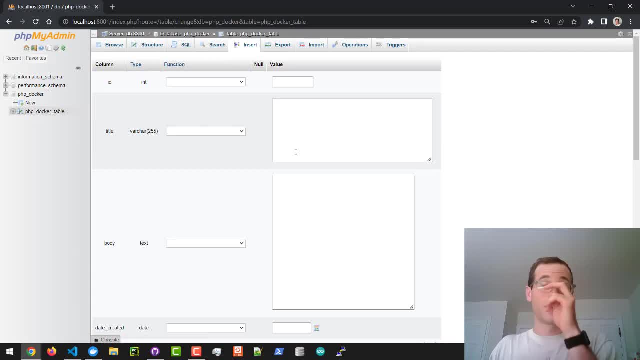 database real quickly. So if I click on this insert tab in PHP, my admin and you don't put anything in to this top row, because this is your primary key and it will figure it out on its own title. I'm going to call this the first title, or you know the first title, And then I'm going to 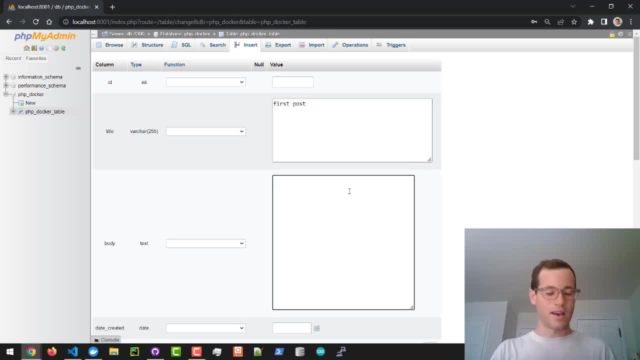 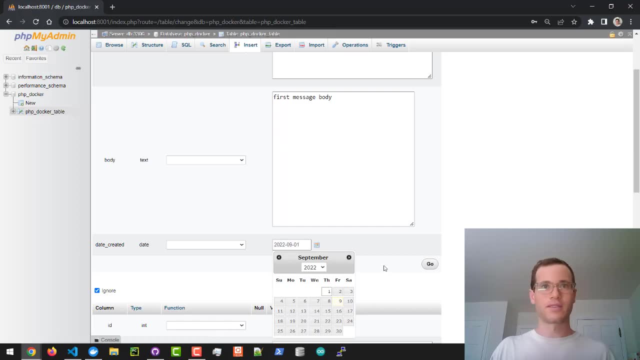 say, you know, first post, just so we use a little bit of creativity And this will be the first message body, just like that. And then the date: I'll say: you know, my first message was last Thursday. And then we'll click on go And you can see that it tells you the actual SQL command: it. 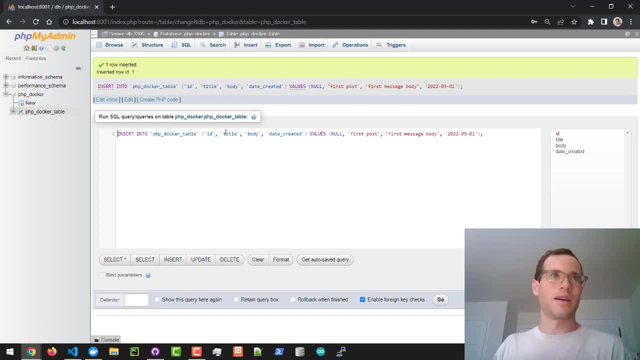 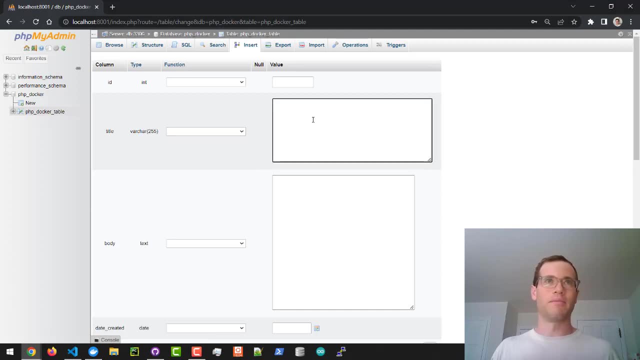 ran in order to make this happen, which is great. I'm going to rerun this again. We'll create like a second little blog post or whatever. So again, we'll call this the second post. And we'll call this the second post, body or message, whatever you want to call it. And then 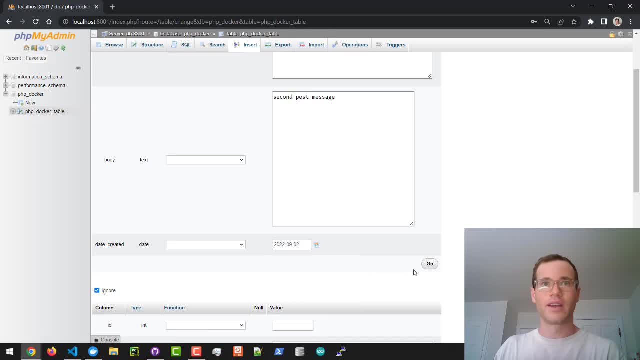 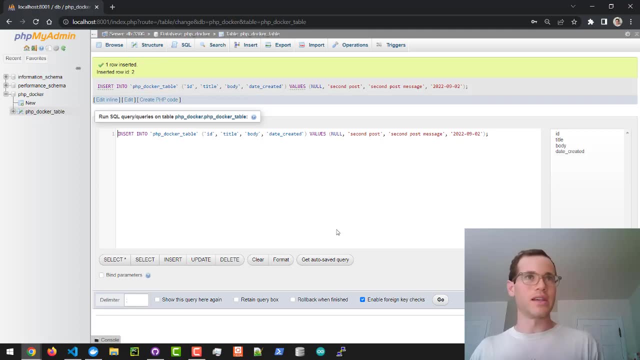 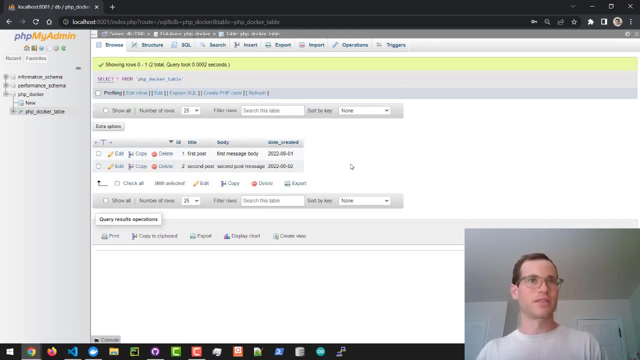 date. we'll say that this thing came out, you know the following day, And we'll click go right there. So we now have inserted two rows into the SQL table that we've created for our web application. I'm going to click on this guy And you can see that it is showing us the two entries. 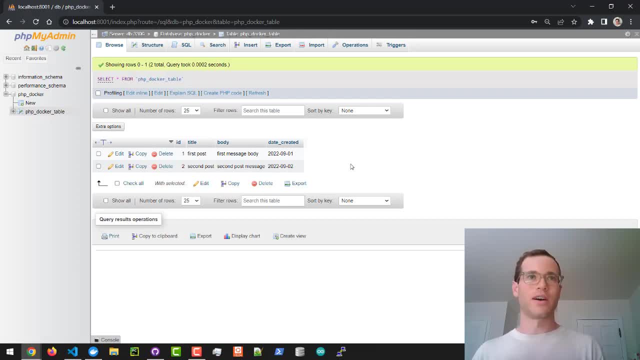 that we've just created. Now, a very important thing to note: when you're creating a web application, you're working with Docker- is that the issue you will run into is that when you stop your Docker container on your local machine, you'll lose all the data. So if you were to stop your MySQL, 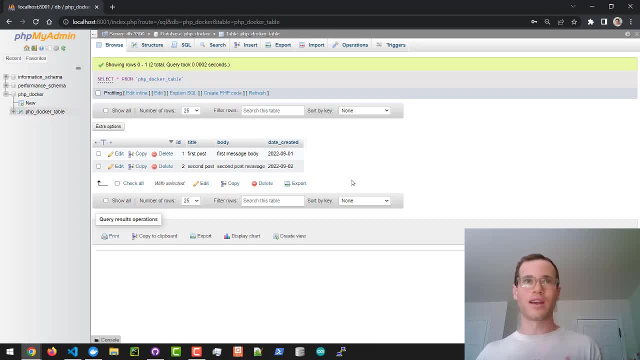 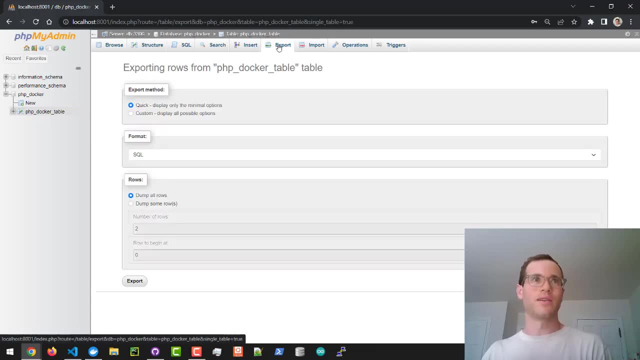 container. right now, these posts that you've just created as your little test will be lost, And so the question is: how do you not lose these? And so what you can do is you can click on export right here, And I'm just going to leave all these defaults. click export again And you can see. 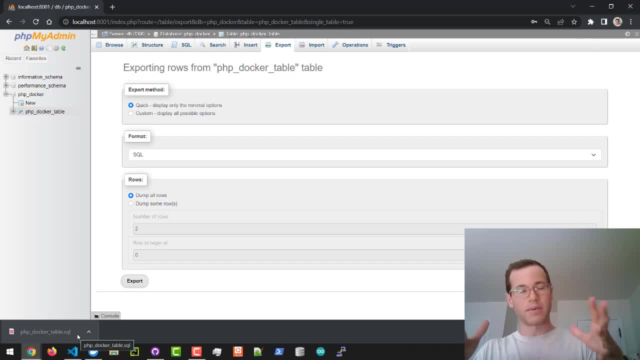 that it's going to download this table, or my, my database, to this little SQL file, And what's happened is that, from the Docker container itself, which is not going to be persisted when it stops running, it has saved that SQL table into my local. 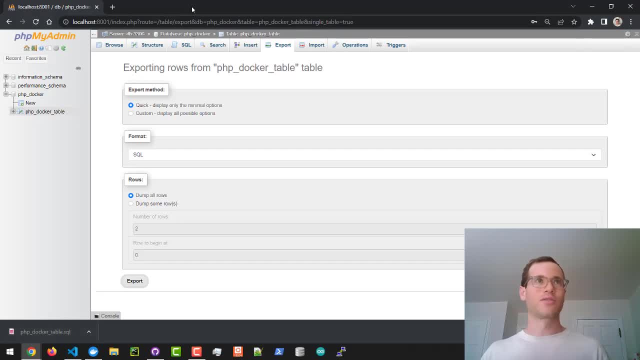 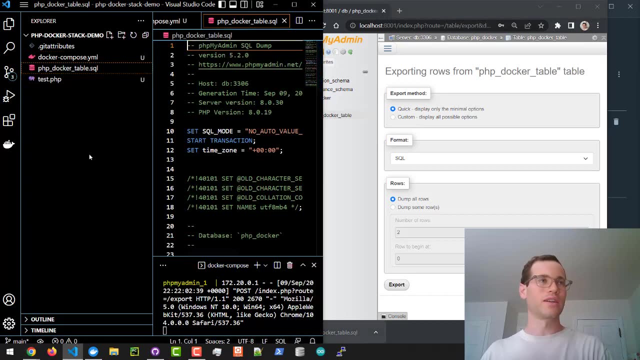 hard drive on this Windows computer, And the reason why that's cool is that if I take this guy and I just drag it or copy it into the project directory of my of the PHP package that's running this full stack web application, is that we now have saved this stuff And you can open it up and view it if you'd like. 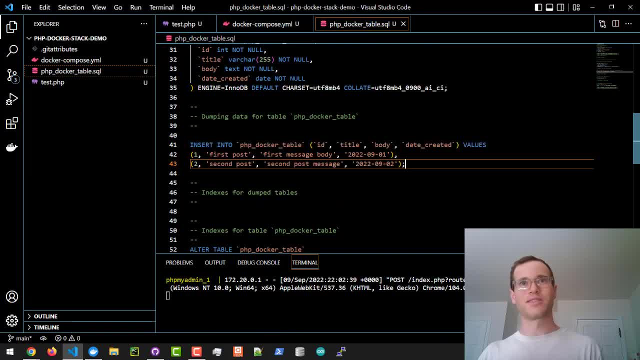 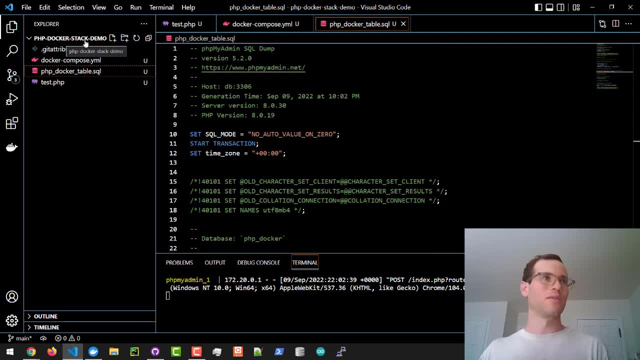 It's really just telling you what it's doing, which is really just inserting these two messages that we've created, as well as defining, like, the schemas for it. But yeah, so that's beyond the topic of this, But what I'm going to do is I'm going to create a new folder right here And I'm 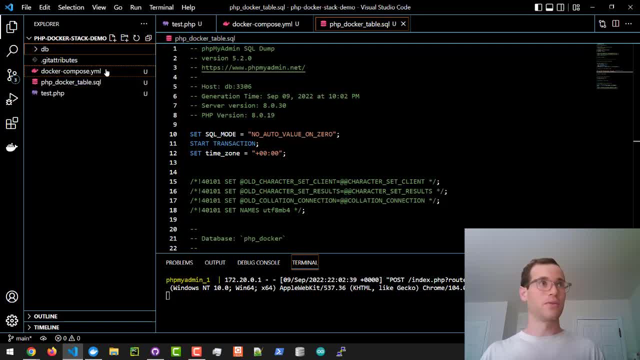 going to call this the database folder, And I'm just going to drag the SQL file into that, just so that we are saving this in a little bit more organized way. So that's what we're going to do, And now that we've done all this stuff, Another thing that's: 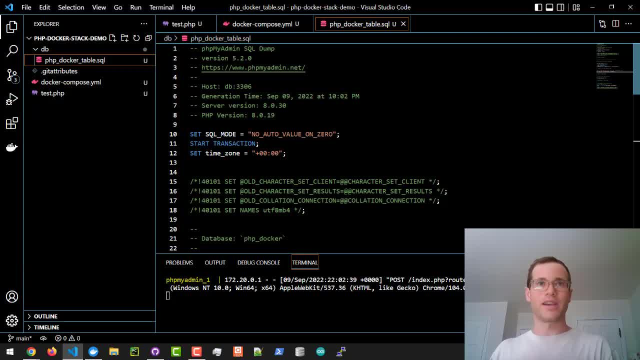 really good to do is, you know, once I stop my container, we're going to lose whatever was currently in there in that, in that SQL service. But we want to reload it. So how are we going to reload? that is, we're going to go back to that Docker compose file And inside of the inside of 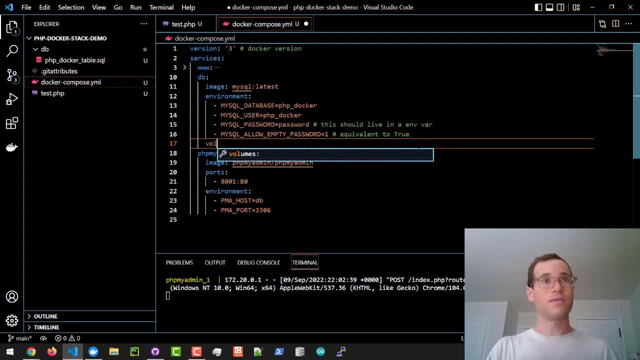 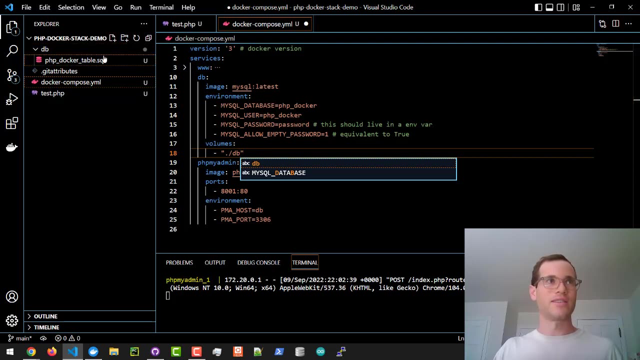 the DB service. I'm going to attach a volume And basically this is stuff that just comes out of the files, from the actual documentation. But we're going to say that you know, whatever is inside my current DB folder that we just created, that now has that SQL file inside of it. we're going to 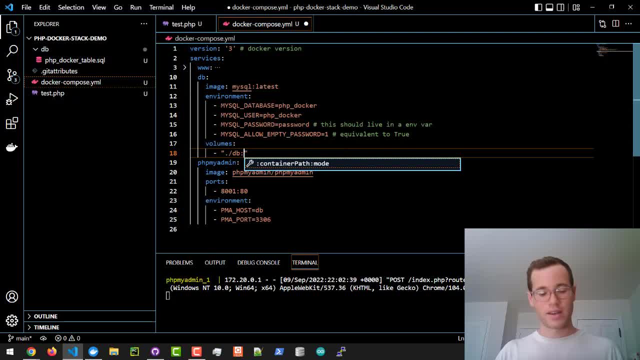 sync that on my local machine with the, with this other folder And specifically what it's called is Docker entry point dash init dbd And this is to sync and this is to sync, and this is to sync persistent SQL files with container. And so I'm going to save this guy And what I'm going to do. 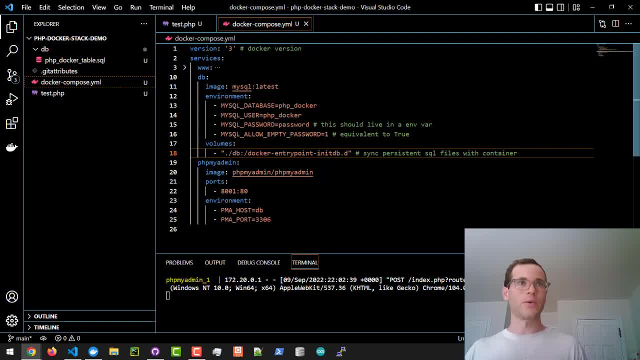 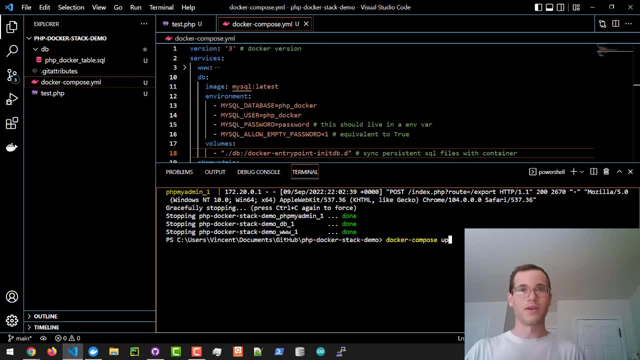 next is: I'm going to test that this actually works the way we expect it to. I'm going to go to the terminal and I'm going to press Ctrl C. it's going to stop my containers. I'm also going to run that. 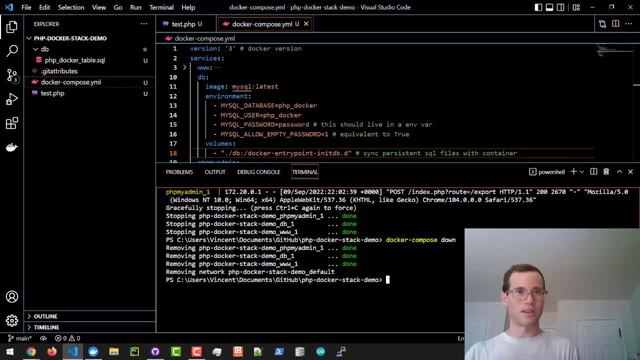 Docker compose down command just to further make sure that we are clearing our resources. And then we're going to run Docker compose up. And this time, when Docker compose up runs, it is going to be recognizing the fact that I've got this little SQL file present inside of my repo, that it should. 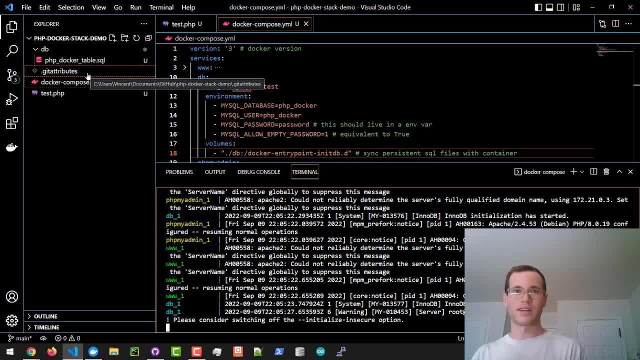 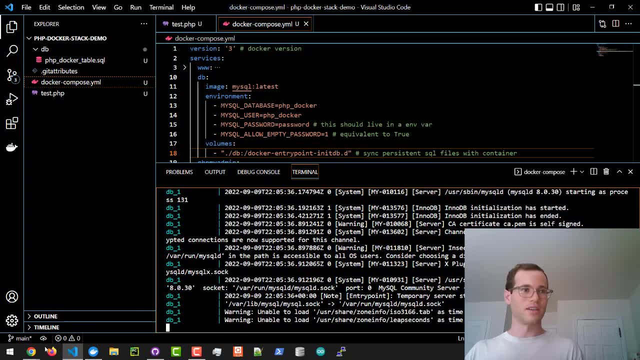 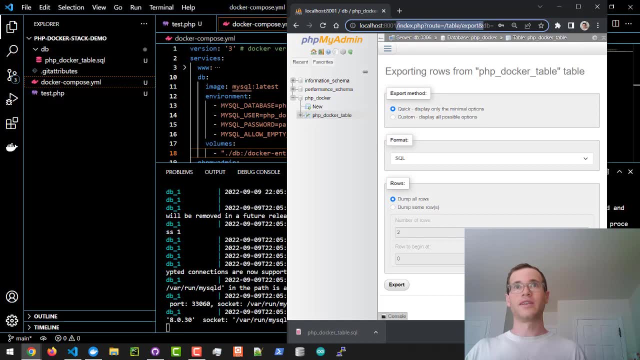 be using when I'm starting this thing up, So I'm saving whatever is inside that database, So I don't have to recreate it every single time. And now what I'm going to do is I'm going to just let this thing finish, But I want to go back to my local host And we're going to go back to port that 8001, assuming this. 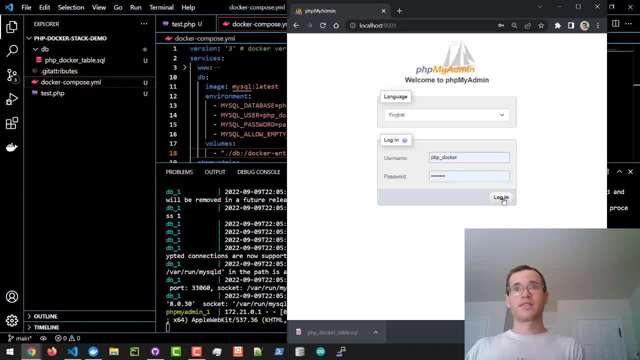 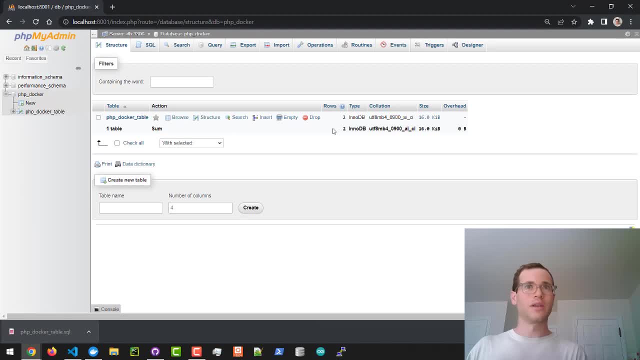 guy's back up in line Run this guy it's gonna ask, asks us to log in. We're going to log in and we're just going to open up this PHP docker table and we should be able to see here that we have. 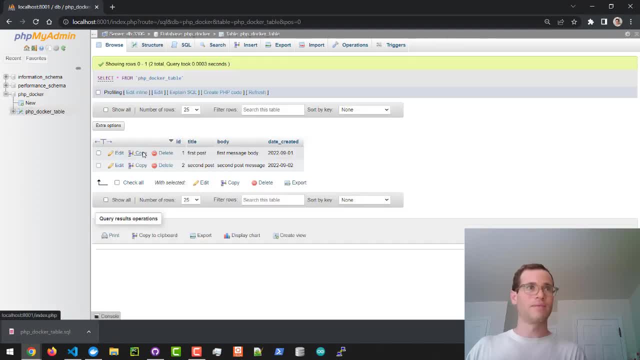 these two rows already in here, So it successfully remembered the entries we've created previously, so that if you are testing this in a dev environment and you want to not have to rebuild your table every single time, very, very useful tool to have. Or if 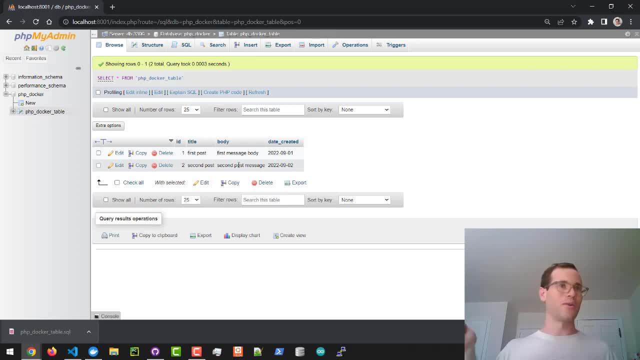 you want to make your application more fault tolerant and handle power outages. this is really really good stuff. to make sure that you are backing this up to, or you're exporting it regularly to, some kind of local disk that will be persisted, like, in my case, this Windows computers disk. So I'm going to minimize 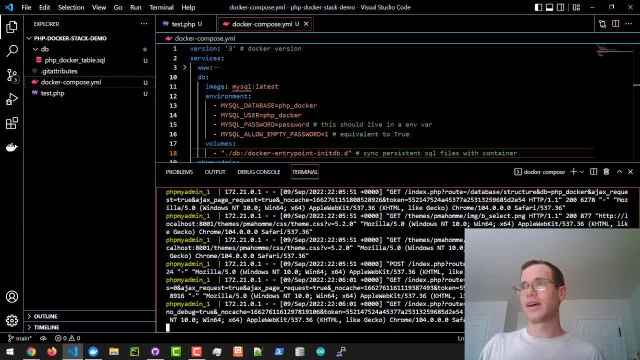 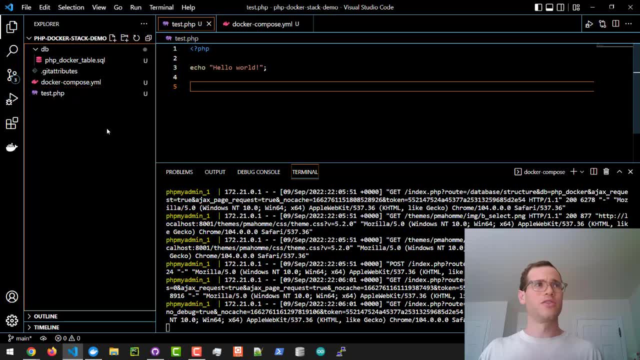 this stuff, and now we are going to work on actually creating a connection to this database that we've created. So I'm going to go back to my project directory. I'm going to create a new file in here. We're going to call this one indexphp. 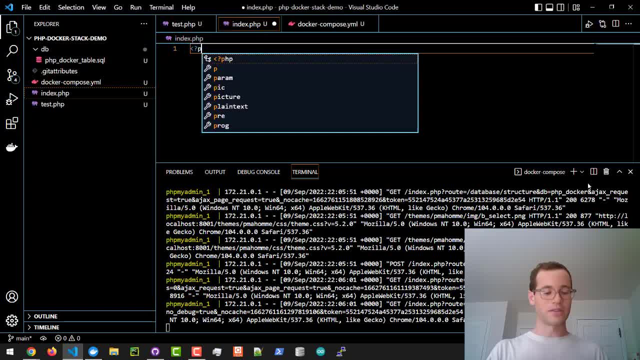 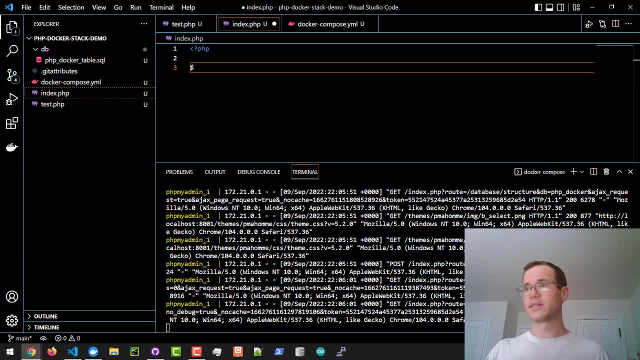 and inside of indexphp. I'm going to immediately start out by defining the opening PHP tag, and what I want to do is I want to connect to the service. I'm going to paste in this stuff because it will be easier for me to explain it. 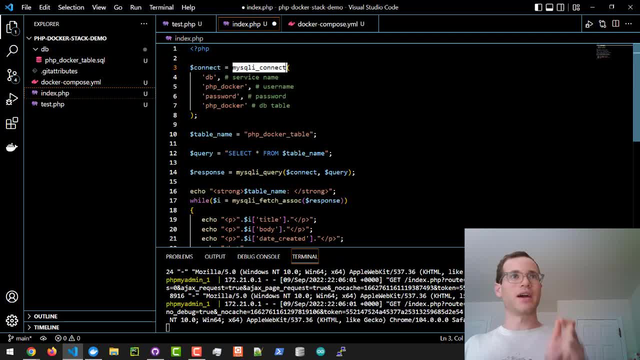 So first thing we're doing is we are calling mysqli. mysqli is a little package inside of the Apache or the PHP container that will allow it to connect to another service inside of our little cluster, and so, specifically, what we're doing here is we're defining this connect object to grab. 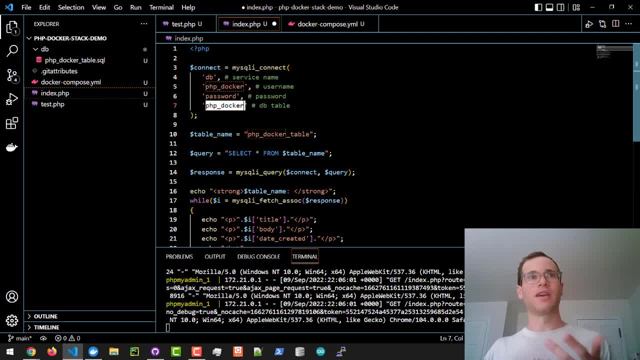 the database and we are passing in the username, the password, as well as the db table name or the name of the database to the mysqli connect class, And so it's going to create this connect object and then from there we're also. 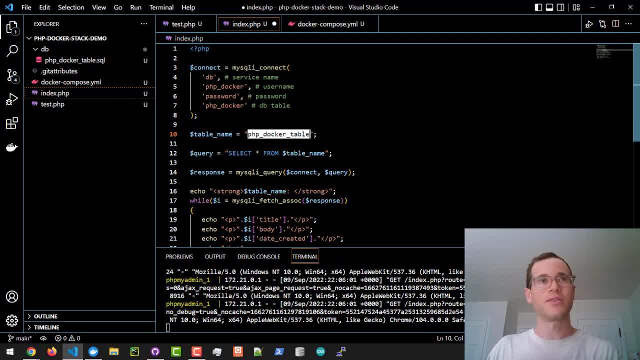 telling it the specific table name that we want to be connecting to, and then I'm going to be running this query. I'm defining the SQL query that's going to be querying this table and in our case, we're just going to be selecting all from this table, so it's going to return us. 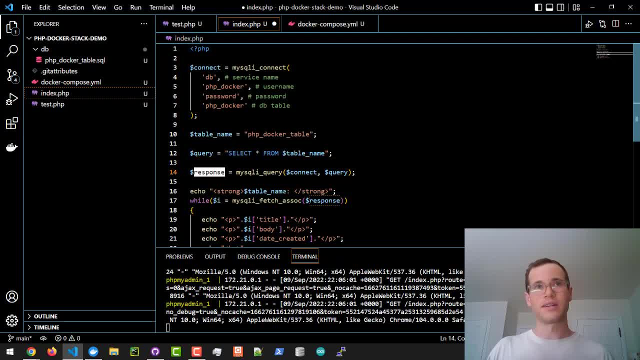 everything and then from there what we're going to have is a response object once we execute that query. so the mysqli package again comes in to execute the query and connect to that database that we have running in our service, and then what we're going to do is: 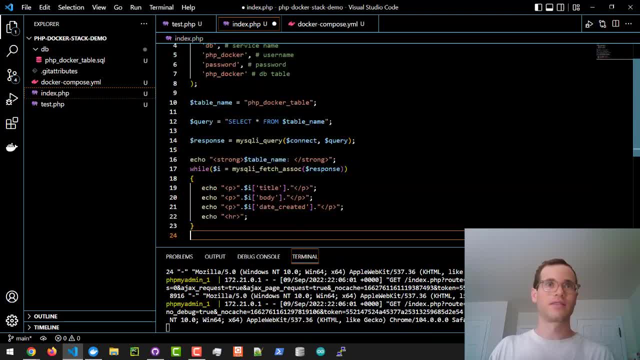 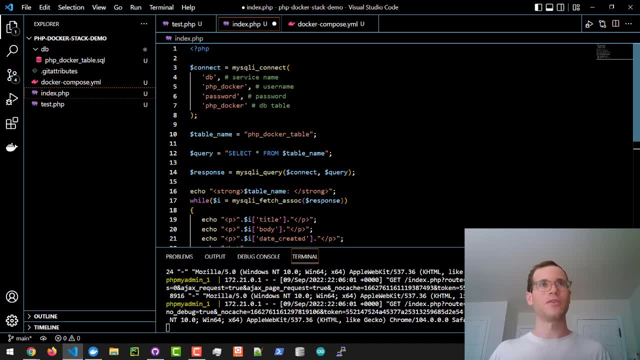 print out all of the items inside of this table and so that's. it's pretty simple stuff, just printing it out. right now We don't have any forms or anything, but you can always add that down the road. I'm going to click command. 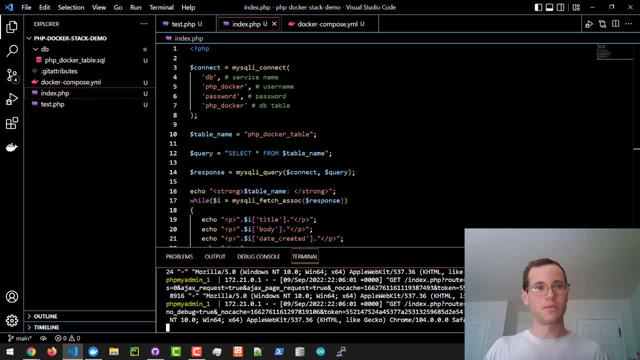 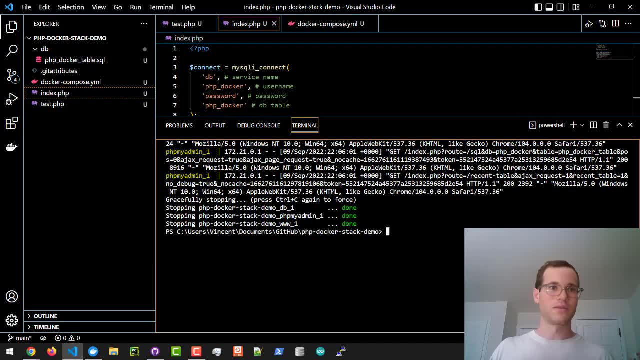 save on the keyboard, and then what I'm going to do is I'm going to just in the terminal, I'm going to do control C just to stop my service and restart this, and so once we've done that, I'm going to run docker, compose down again, followed by 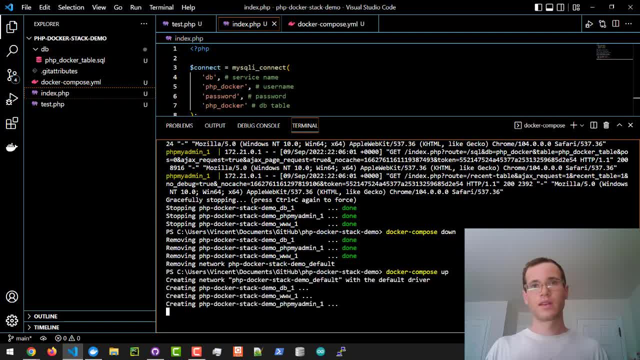 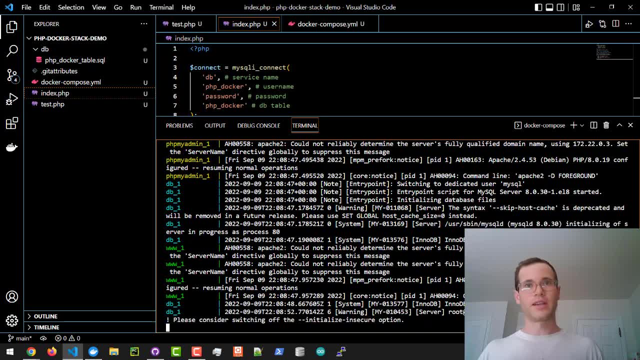 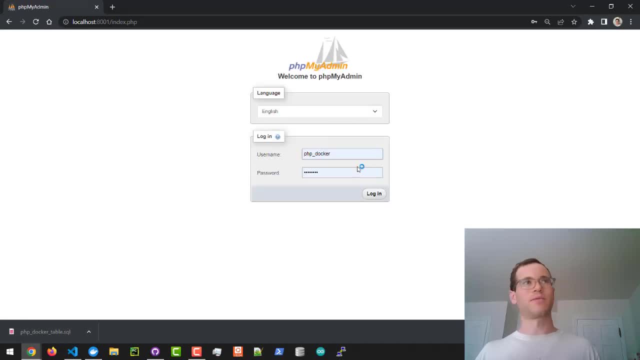 docker compose up. Okay, And while this thing is booting back up, I'm going to open up the chrome tab I have again and I'm just going to go back to that mysqli admin page to confirm that our service is running again. so it might still be booting up, so we might have 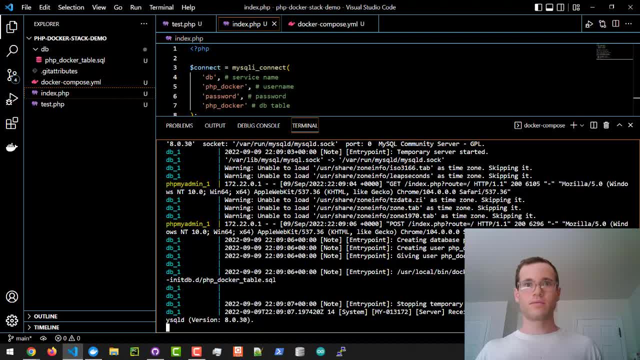 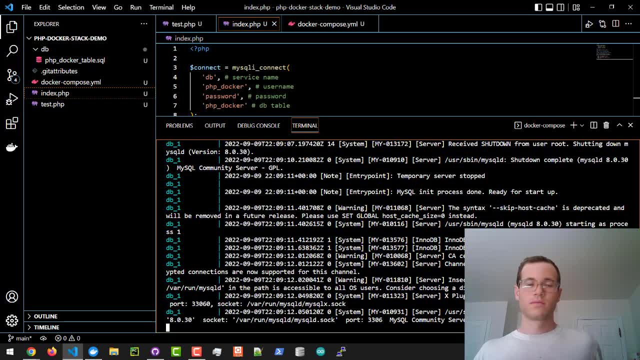 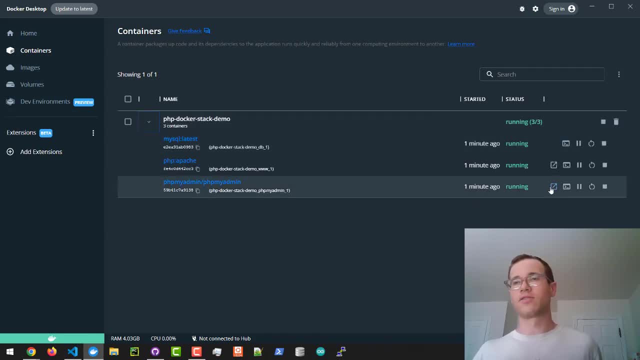 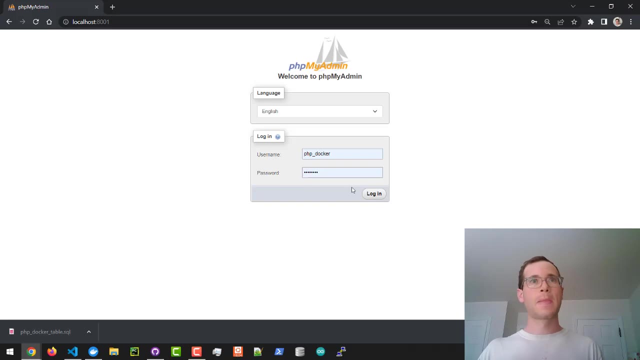 to give this thing a little bit more time. Another thing you can do to check is if you open up the docker desktop thing, you can see in here that it says it's running, back running. but I just want to see what it's telling us all right, so now the server. 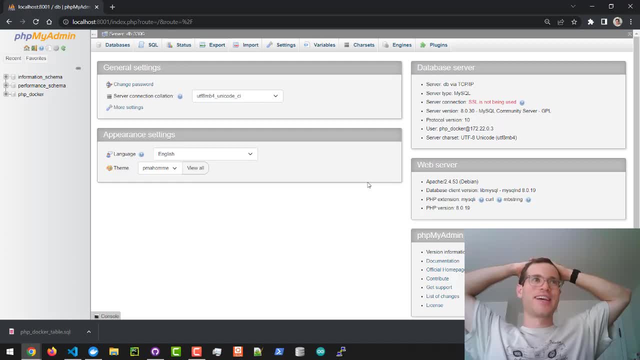 is up. I didn't do anything, just was a little bit more patient. but now we've got our database running and what I want to do is I want to go back to the local host and we're going to go to indexphp and we're going to run into this. 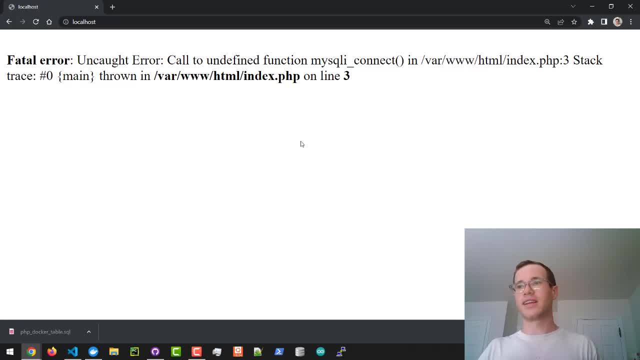 error message, which is a pain in the butt to deal with, but this is part of learning. so, basically, the issue is that the mysqli package is not yet installed inside of the container that is running the PHP code or the PHP service that we need. so the way we resolve this is we are going to go to docker desktop and 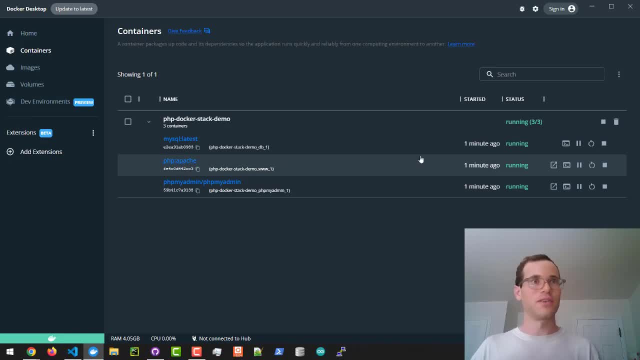 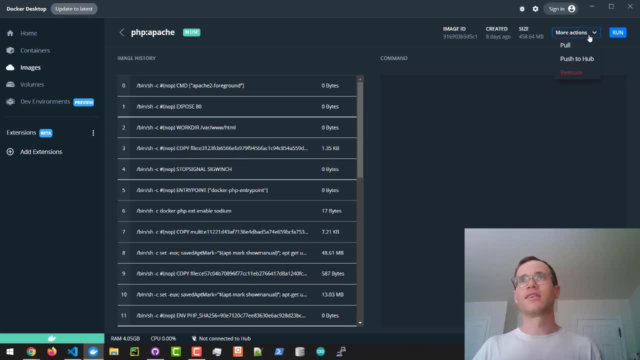 we're going to view the PHP service that's running and they have this little button here that says so. if you click on this guy, they should have you. there's a spot where you can open this up in the in the command line, so you can see exactly what's going on. 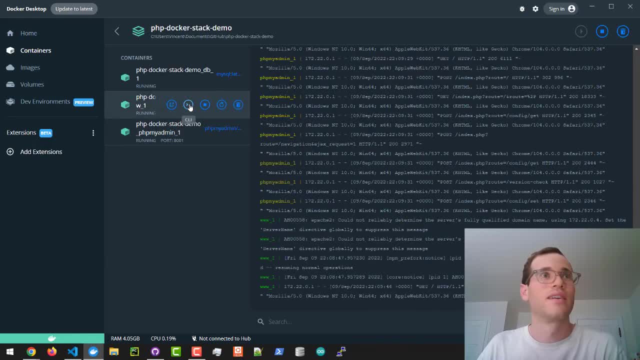 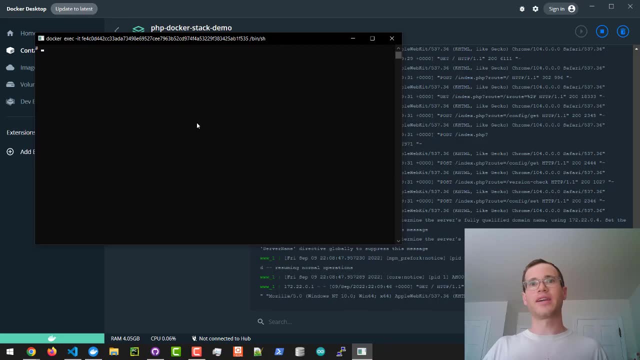 and I just want to get to that one second, run this CLI. so what this did, is it just opened up a CLI connection, or well? I'm now viewing the CLI, the command line interface of the docker container that is running the PHP service, and, And what I want to do is I'm going to run this command: paste that guy in. 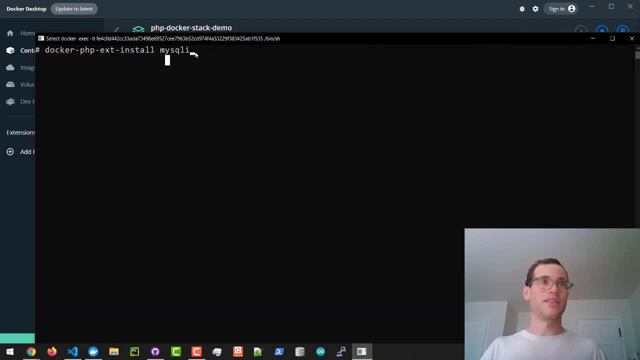 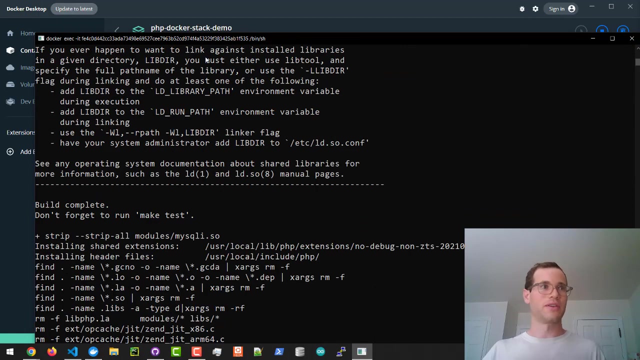 So what this does is it is going to install the MySQLI package that is needed to actually make all this stuff run, because MySQLI is needed to allow the PHP that we're running to actually connect to the MySQL database that we have, And so we're just going to let this thing go through its song and dance and it looks. 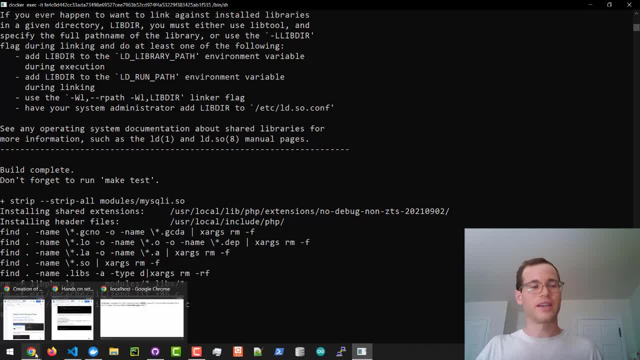 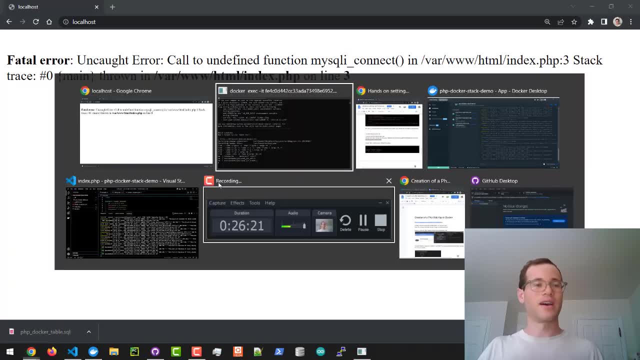 like it's successfully installed. So now that that is the case, I'm going to go back up to here and we're going to refresh this page, And it still might not work. so what I would recommend doing in this situation is I'm going. 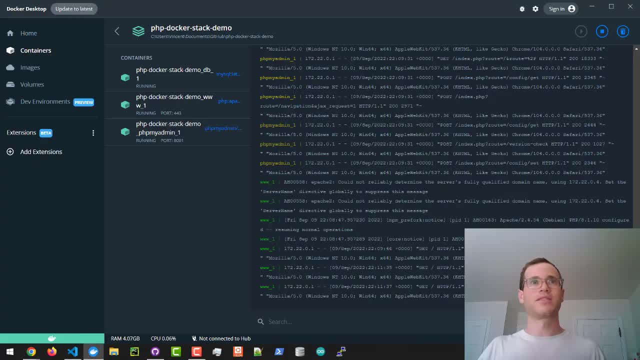 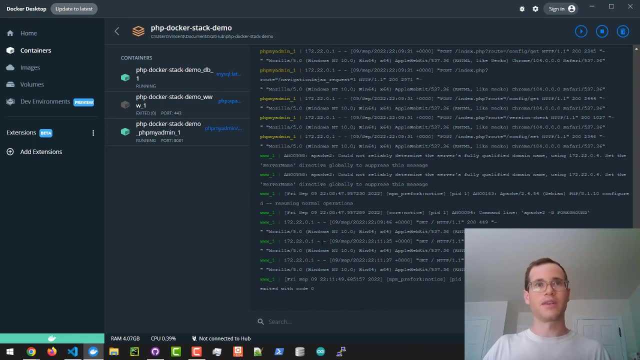 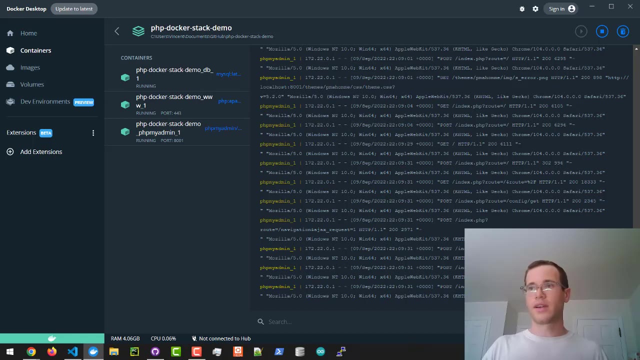 to close out of this interactive terminal. I'm going to go back to the Docker desktop and I'm going to restart this specific container and we'll give it some moments to finish rebooting. Okay, And my, It might be a little bit premature, but we'll see. 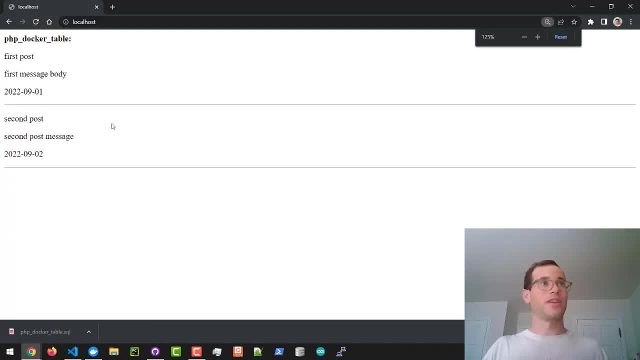 So I'm going to go back to here, I'm going to click on refresh And now that we've installed the MySQLI package inside of the actual container by going to its command line interface and we restarted that Docker service, we are able to view the 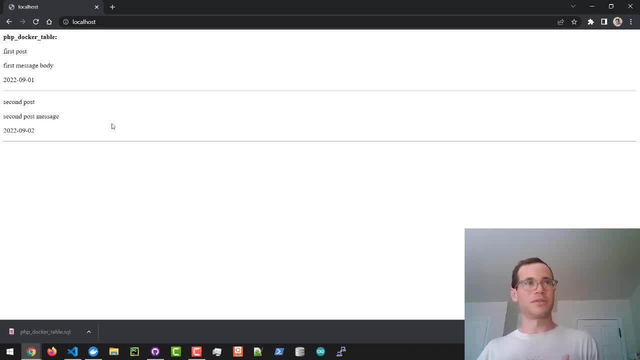 contents inside of our actual MySQL table with PHP. So basically, what we have done is we have just created a full stack web application. It's all written in PHP And it is showing us the contents of a database in a separate service, And so we now have a back end as well as a front end for us to play with here. 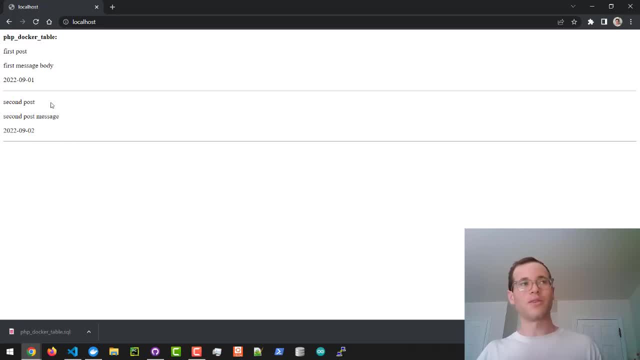 And it is showing us the dates, the body of the message, the name of the message, And so, just like that, we are off to the races, which I think is pretty awesome stuff. I will be posting all this stuff to GitHub so you guys can clone this repo and run it. 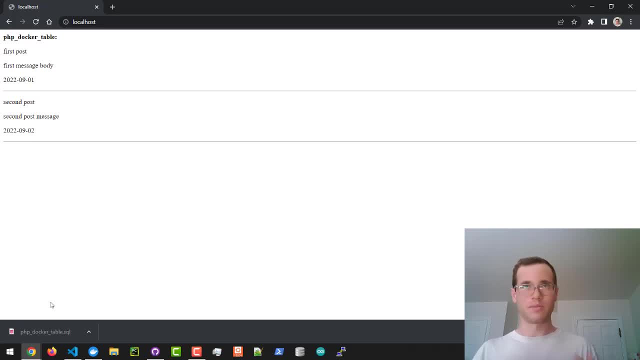 And just as long as you run the Docker compose file, you should be able to have a starting point to start developing full stack web applications, Which I think is really awesome. So thank you all for watching. Let me know if you have questions and I will talk to you guys next time.